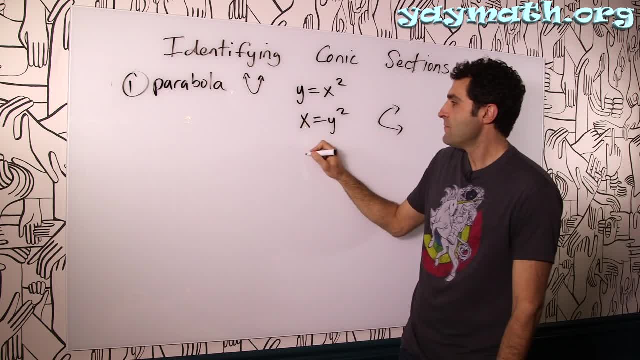 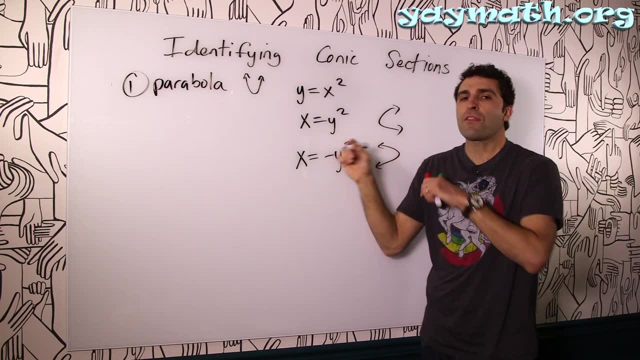 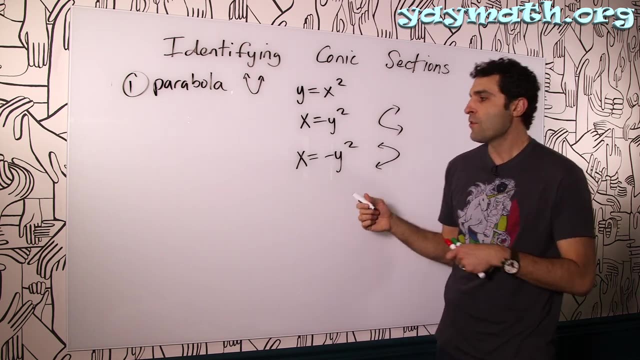 facing right. If you had x equals negative y squared, that in turn would be the parabola facing left. So no matter what throughout the equation, no matter how you slice it or dice it, you will never see both. So that's the conic of the variables squared. So a lot of times in the books they'll say: 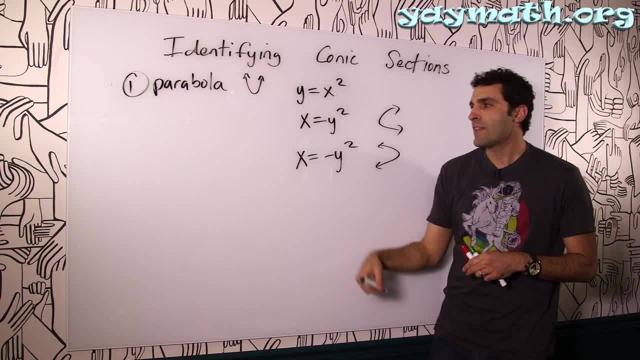 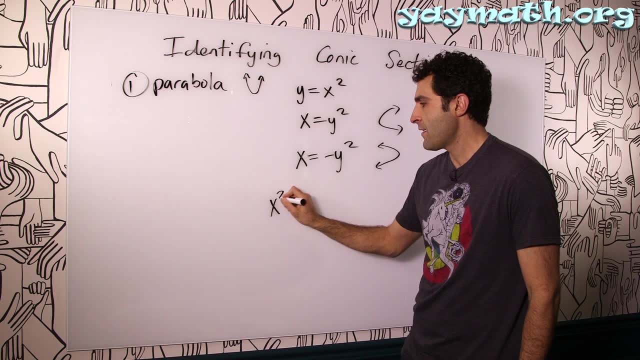 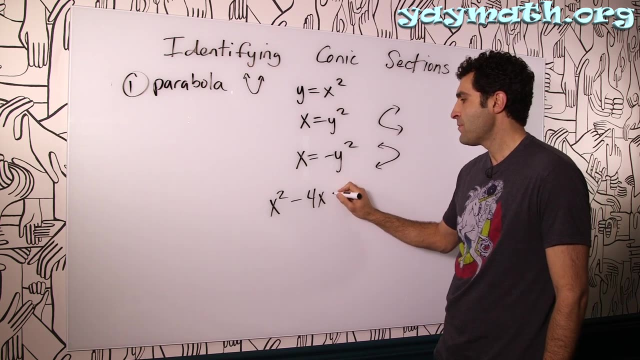 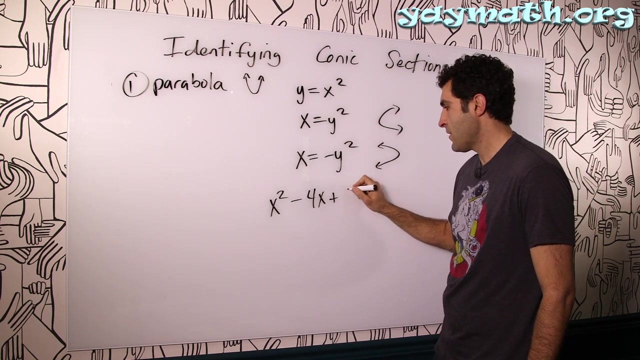 identify the conic and then write it in standard form. So let's throw out a possible example. You could see something like: let's say it was x squared minus 4x plus 2, whatever equals – how about minus y? That'll be fun. Plus 2 minus y equals 2.. 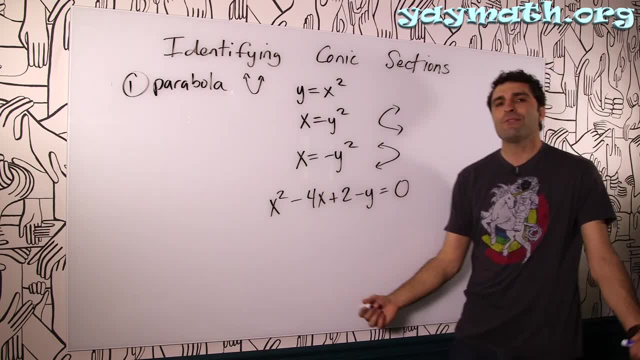 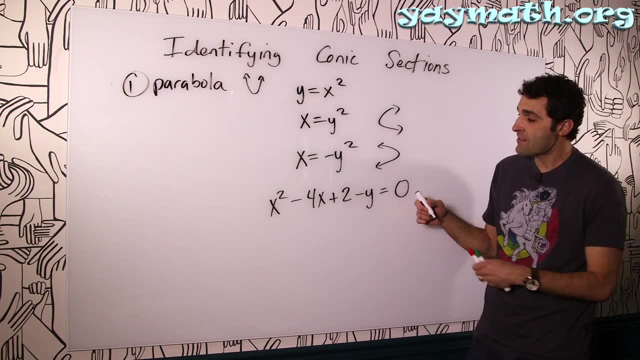 Plus 2 minus y equals 0.. See again, this is the idea. You're looking at that thing, you're like, I don't know what that is. But the second: we know what to look for. in which only one variable is squared, we instantly know it's a parabola. In that case, it is. 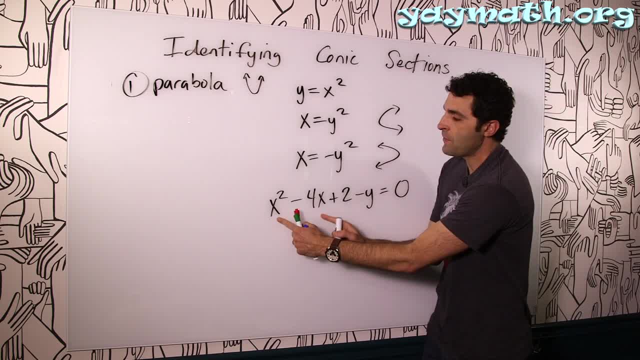 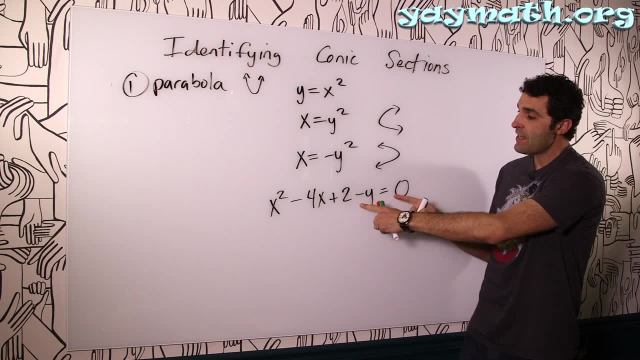 a parabola, because we notice that the x value is squared right, So these two will be paired And the y is not. so this is a parabola, So we're going to put it into this standard form in which one of the variables is isolated. 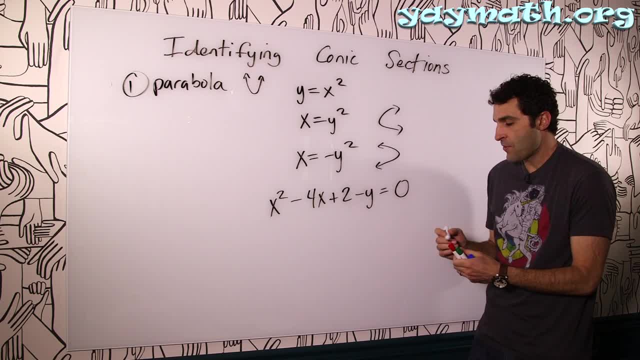 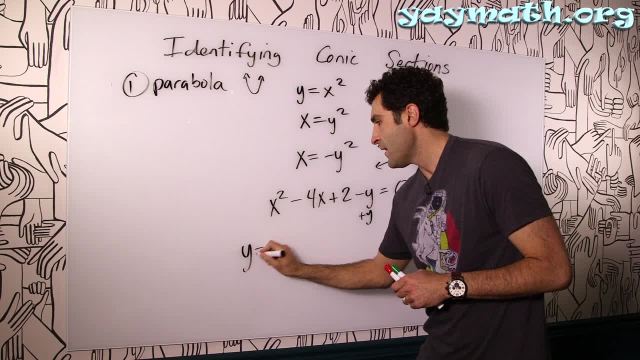 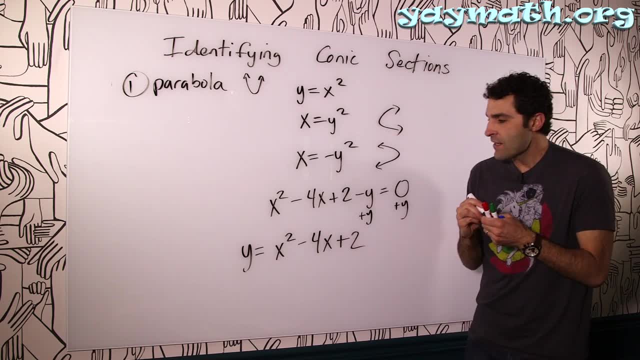 Okay, Okay, Okay, Okay. Just going to write it on the left now. So you get y equals x squared minus 4x plus 2.. So it's not in standard form. So get ready, Hold on, Saddle up. It's time for completing. 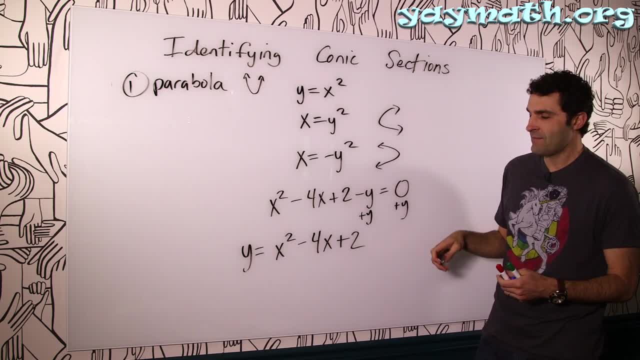 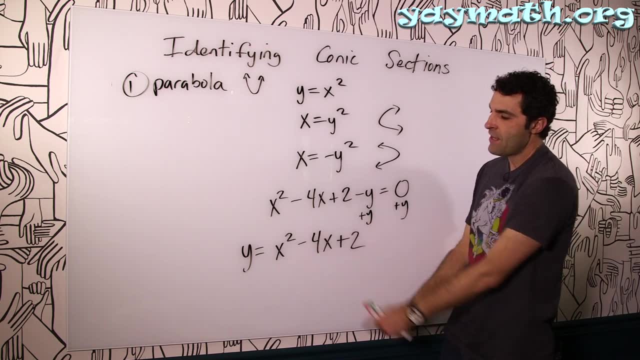 the square lifestyle. So here's the dish, the the dishu. I'm going to dish out the issue. Here's the dishu: We can't complete the square. We can't create a factorization of x squared minus 4x plus 2.. So what many students like to do is they like to move this. 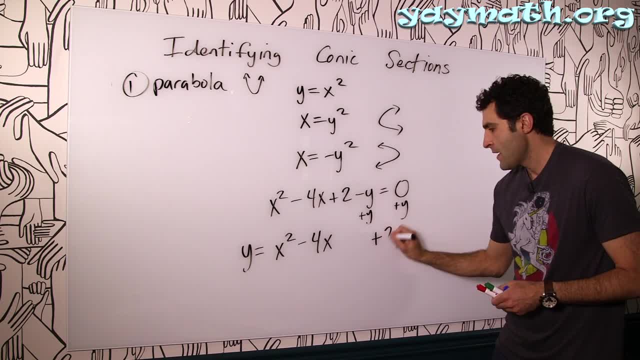 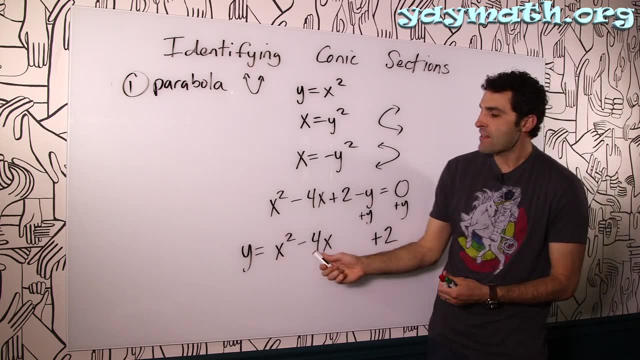 to. you know, a modal variable. So you can't create a factorization of x squared minus over to the right. put it over here. we ask ourselves: what would this value have to be such that this can be factored? okay, there is a process to it. I'm gonna. 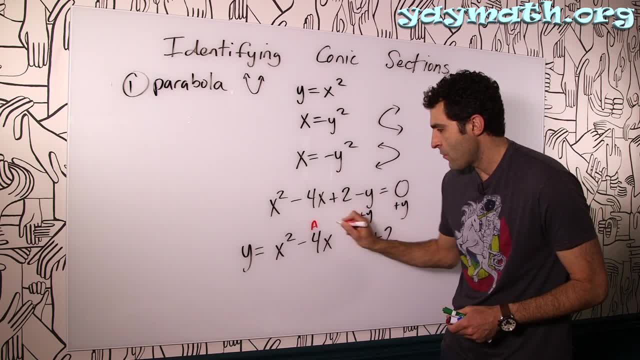 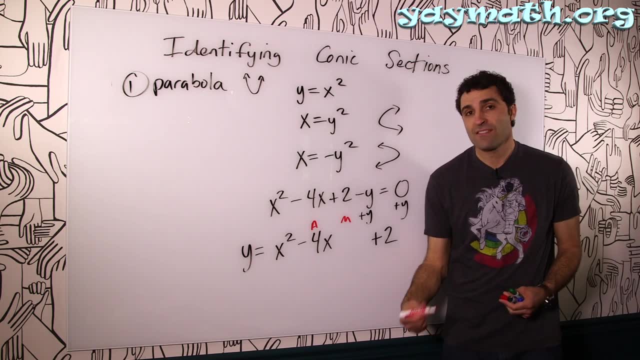 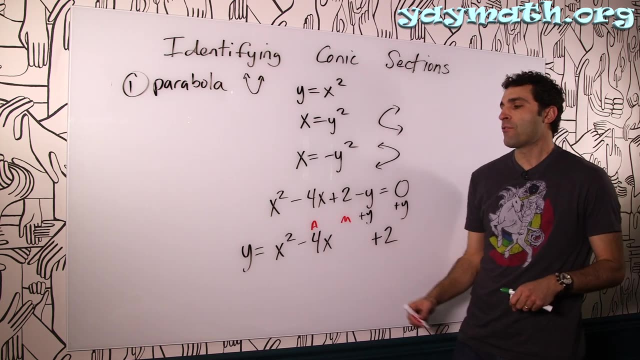 give you that process in just a second. but essentially we're looking for two numbers that multiply it to some mystery number and add to negative 4 in which those numbers are the same. so this is the giveaway in your detective game: what two numbers would add to make negative 4 in which those numbers are the same. 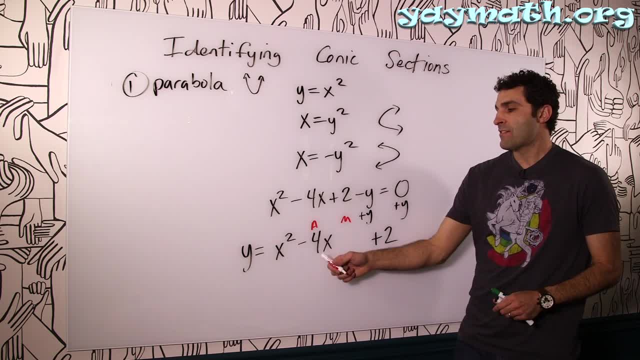 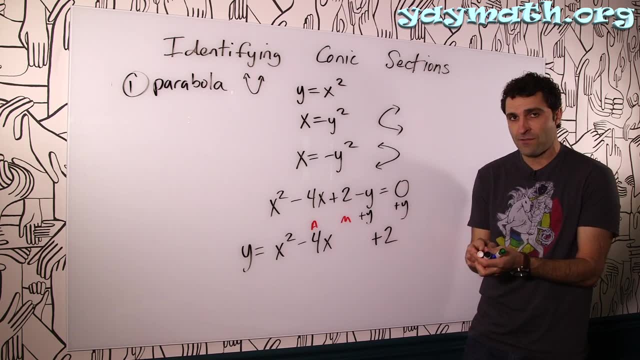 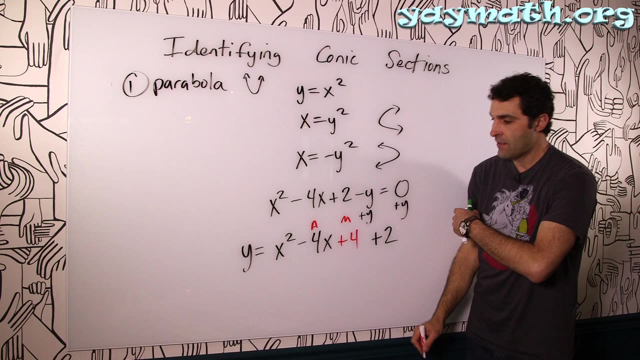 those numbers are negative 2 and negative 2. we know that. and so if those are the numbers- negative 2 and negative 2- what do they multiply to make? they must multiply to make positive for negative 2 times negative 2, positive 4. so we're going to add 4 here now. according to the rules of algebra, this: 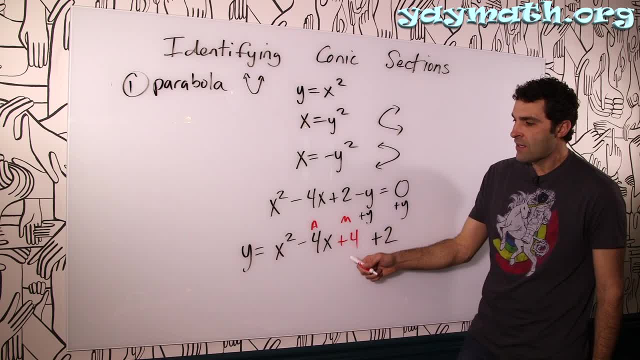 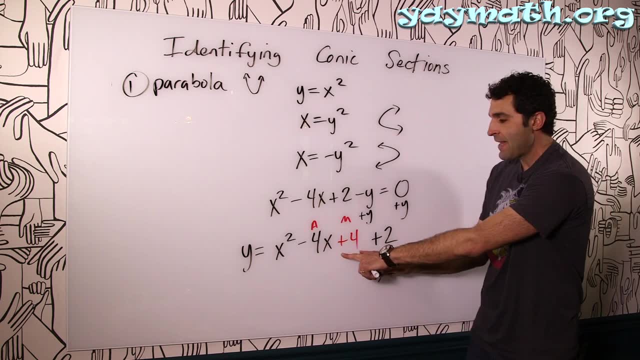 equation requires balance. if we added 4 to this side, we're required to add it to this side as well of the. but once you get going you become a pro at this stuff. I'm allowed to simply go plus 4 minus 4, right, so that had no net change to the equation. that's sort of. 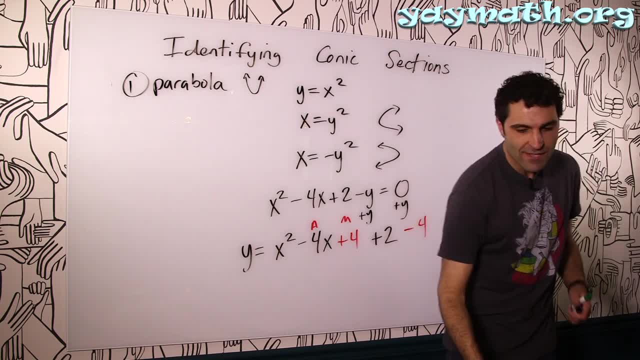 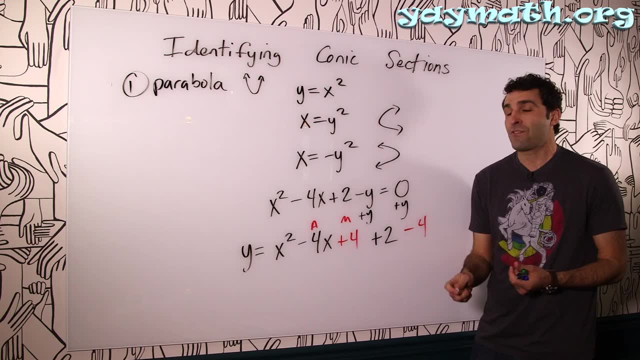 like if I take out four dollars of my wallet, put it on the table and then pick it up again. it's like the same concept and there was no change to amount of money in my pocket, except for the scare of losing four dollars. so let's go ahead. 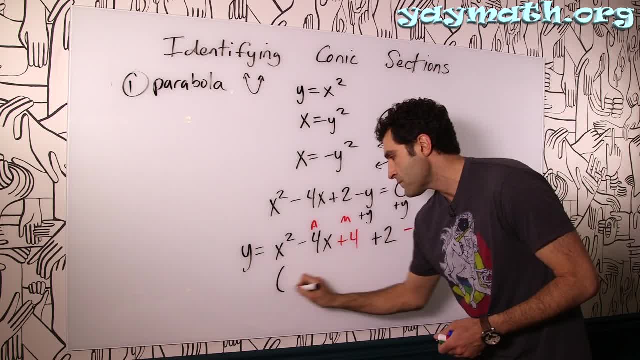 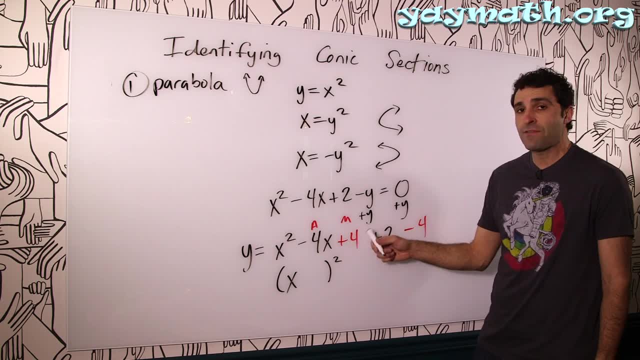 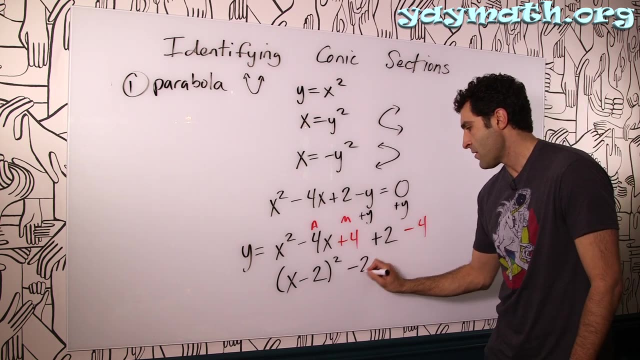 and do this. this now factors 2. all right, what two numbers add to make negative 4 and multiply to positive 4? those numbers were negative 2 and negative 2. there they are, and then this happens to add up to negative 2 as well. right, that's a. 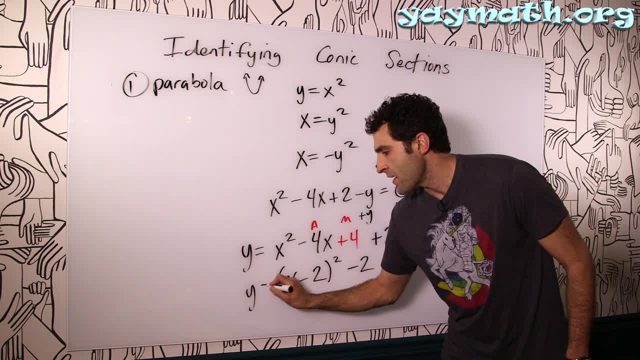 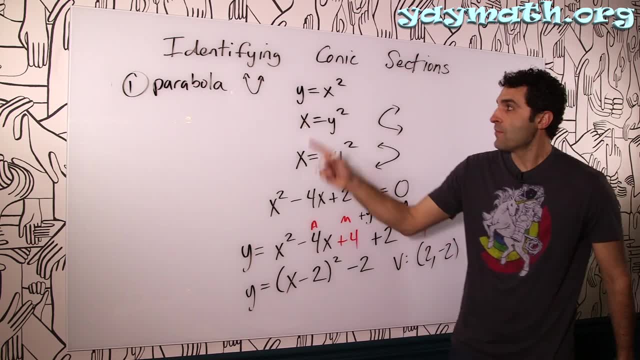 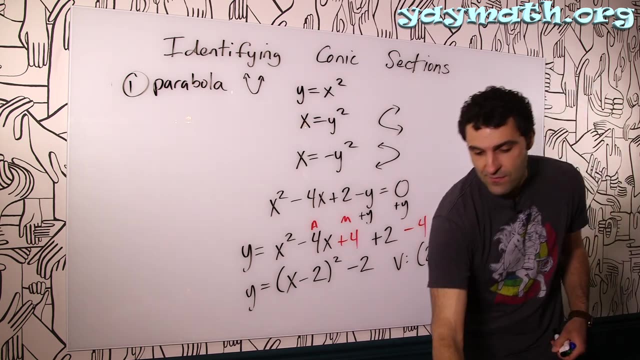 total coincidence. and so here's your equation in standard form. all right, this vertex is that 2 negative 2 and this problem faces up. that's that one. all right, so that's the first one. it's a parabola when only one of them is squared, one of the variables 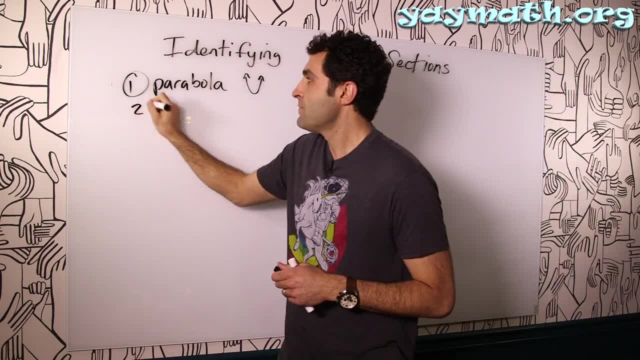 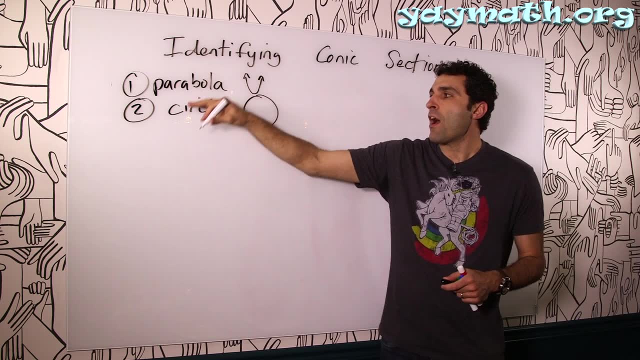 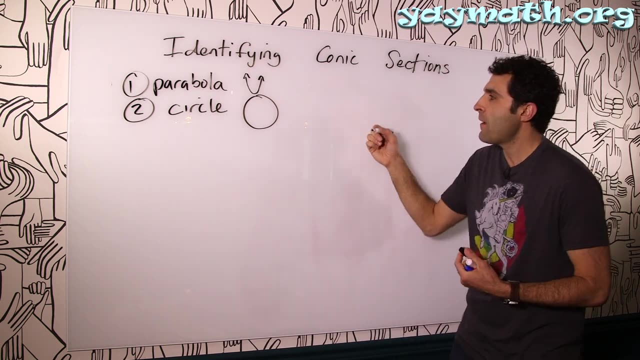 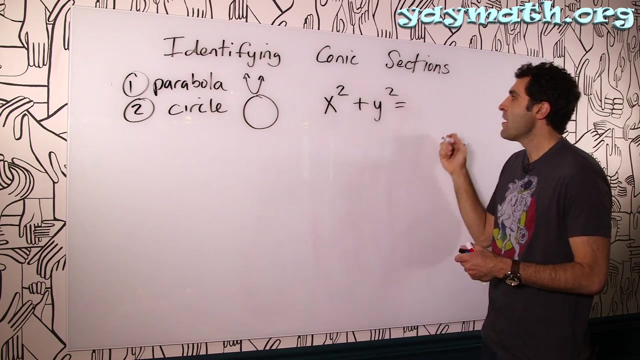 so the next one is the circle circle coming up. okay, so from now on both of the variables will be squared X&Y. the question is how and what it looks like. so the circle is a very straightforward formula. it's pretty much this: X squared plus y squared equals. let's put down like 16 as an example. So you'll. 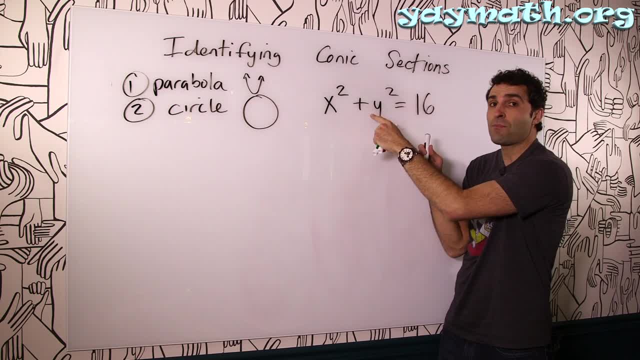 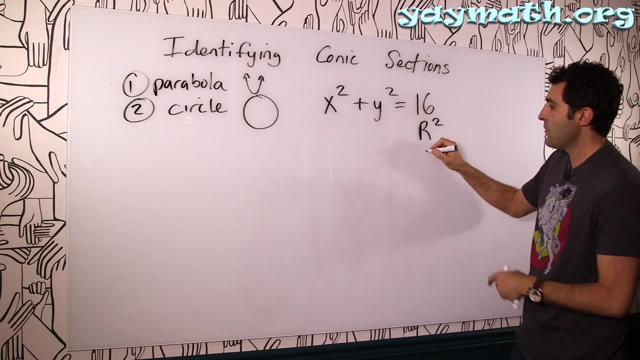 notice both x and y are squared, You'll notice that there's a plus between them. That's important, And this is the radius squared. So if this was r squared, that would lead us to conclude that r equals 4.. The radius is 4.. Alright, So you'll. 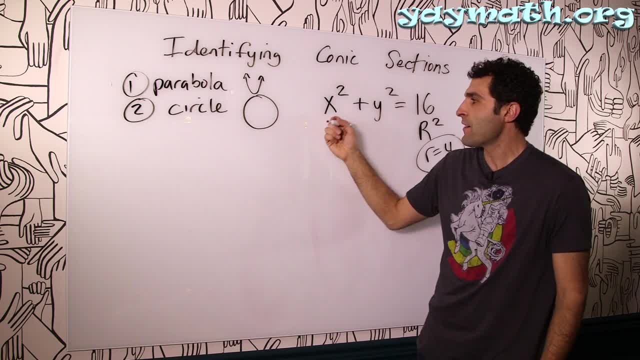 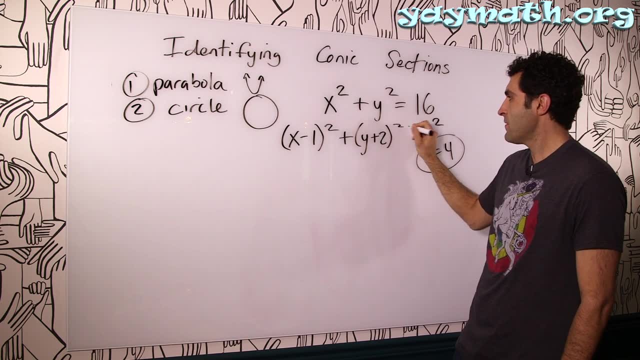 notice both of them squared and the radius is 4.. It doesn't matter how you slice it. This could be: x minus 1 squared plus y plus 2 squared equals some sort of other radius. Let's put 16 again, Why not? So the r is still 4.. This is still a. 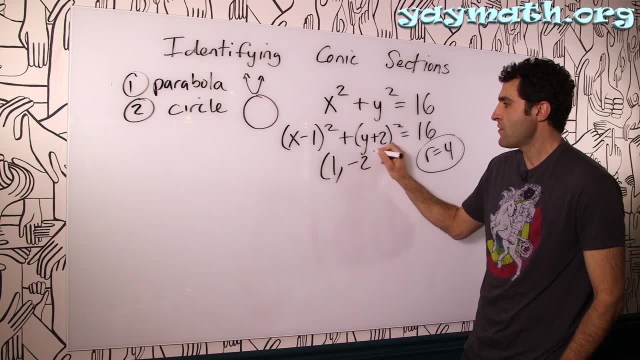 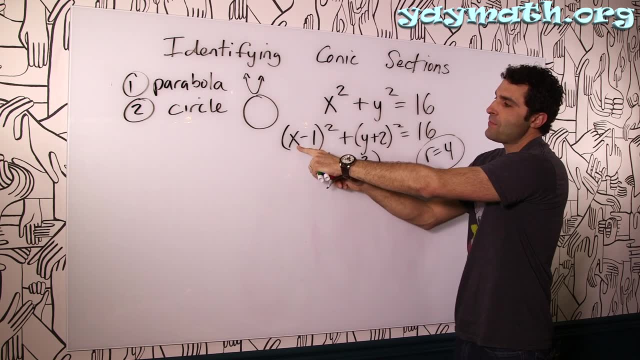 circle. The center is 1, negative 2.. You'll notice this opposite effect, similar to what we had within the square of the parabola. You get this opposite effect because 1 minus 1 makes this go to 0. So that's the center point. So the center is: 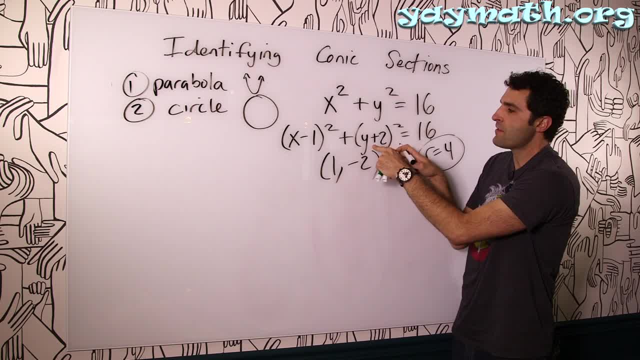 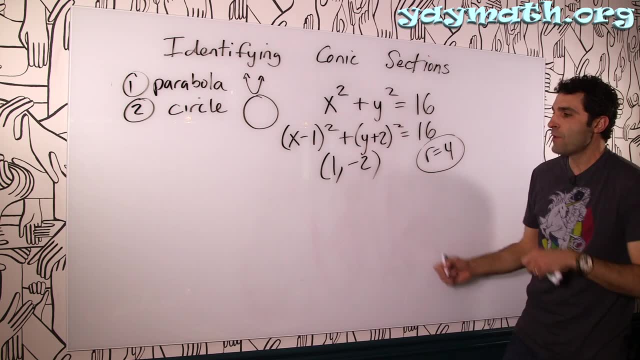 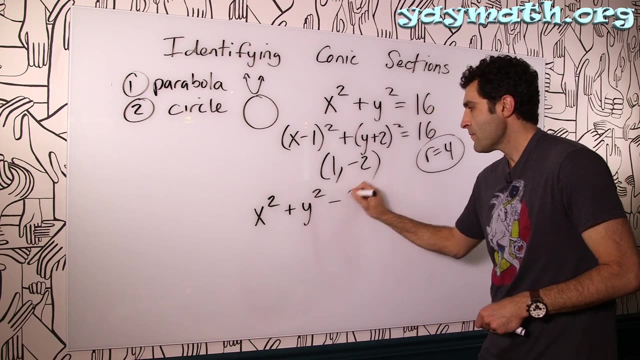 at 1.. Opposite of negative 2 here is, excuse me, opposite of positive 2 is negative 2.. And then again, this is radius squared, so the radius is 4.. Alright, So that's the giveaway. A simple example would be like, let's say, x squared plus, y squared minus. 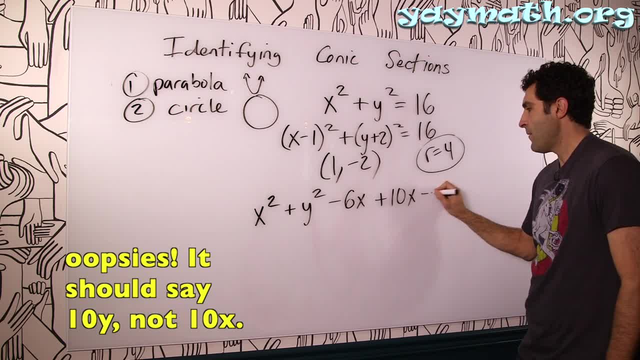 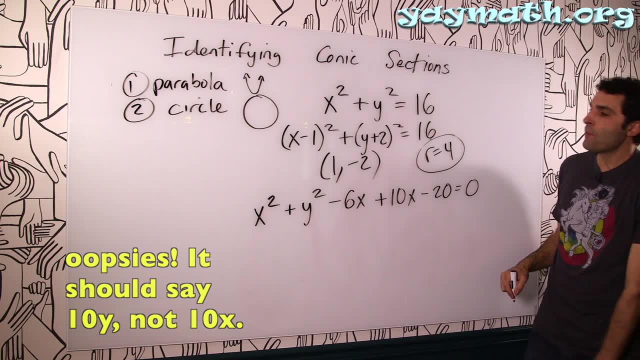 6x plus 10x minus, let's say 20 equals 0.. Again, at first glance looks intimidating, But we notice x squared and y squared are both squared. x and y are both squared and there's a plus between them. So we're. 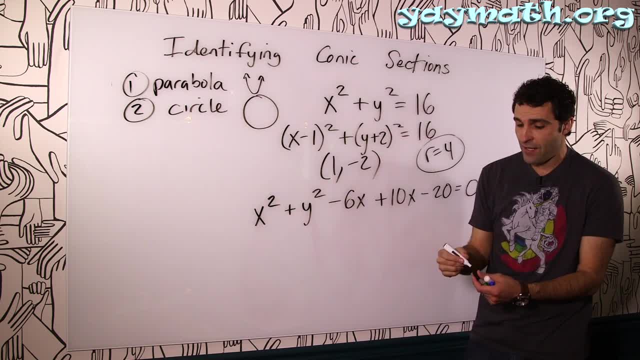 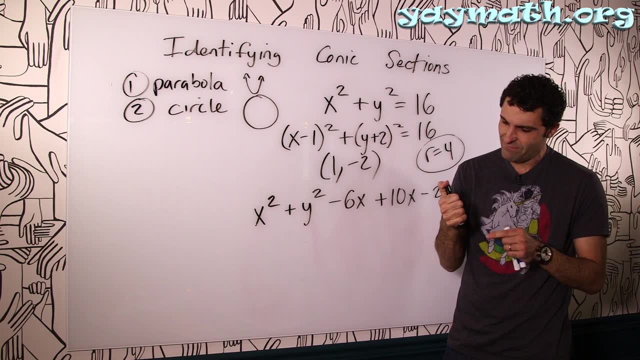 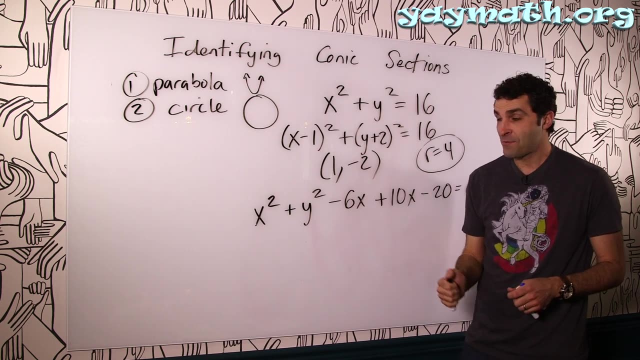 automatically thinking circle. And another thing is that we notice no coefficients out here. Note: this marker is very new. It's like, ah, satisfying, Very new markers. I like to fidget. That's what I do with my hands a lot. It helps me think, So you'll notice no coefficients. 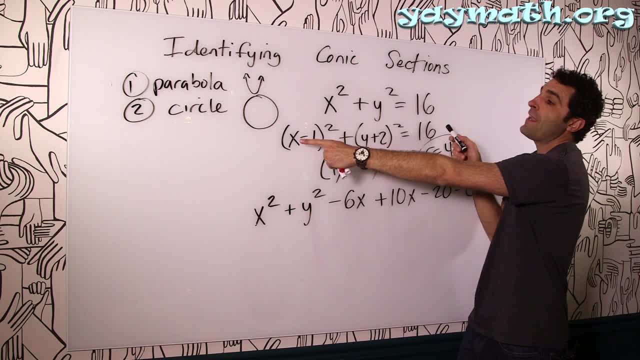 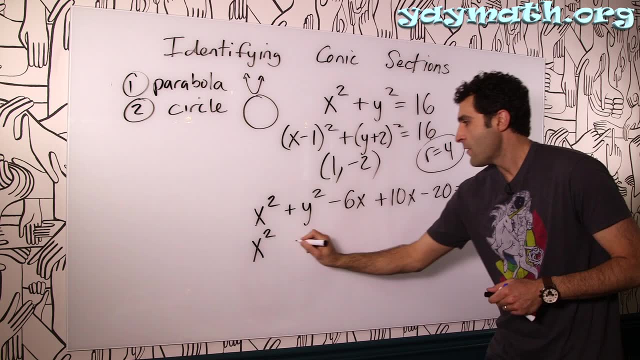 out here. So that's the giveaway: that this is immediately a circle. We want to make it look like this. So, again, we're going to do a little, completing the square party. So let's group our x's. We've got x squared. We've got minus 6x. Leave a space. We've got our plus y squared Plus. 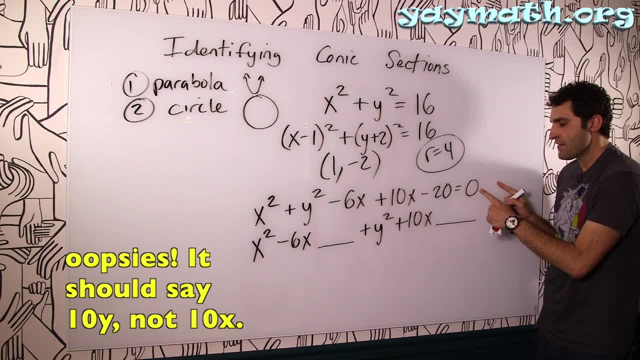 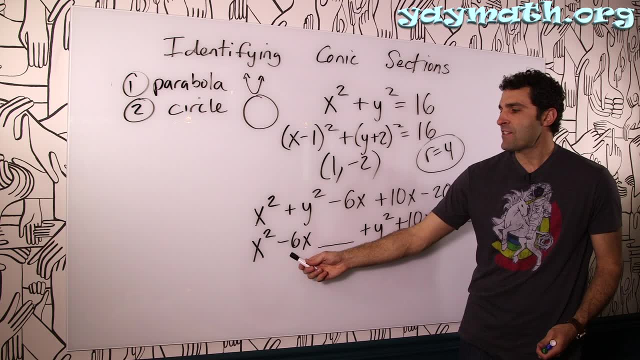 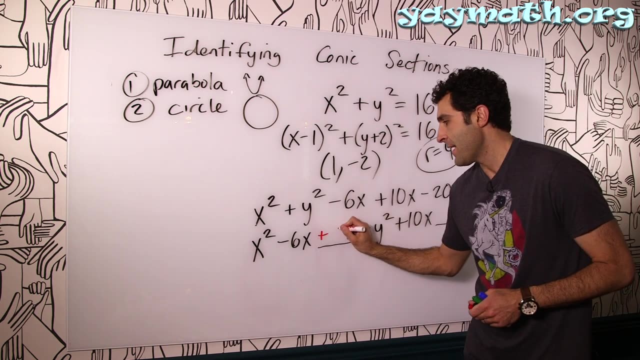 10x. Leave a space, Add 20 to both sides, So it's going to be equal to 20.. Great, So let's complete the square Numbers that add to negative 6 and multiply to blah. So those two numbers must be negative 3, negative 3.. So this would be a plus 9.. So I'm going. 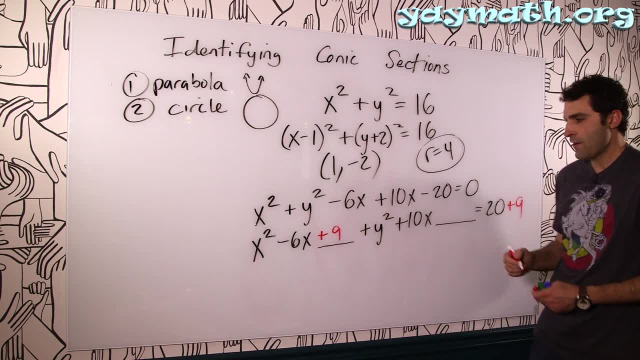 to add 9 here and I'm gonna add nine here. all right Again. so I did promise you that there is a process for this. The books offer this process and it's fine to use it, as long as you understand the context. 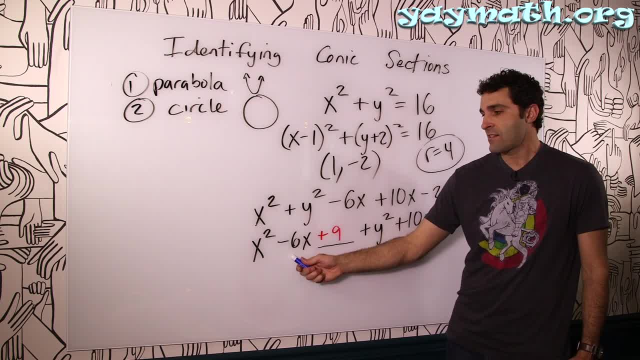 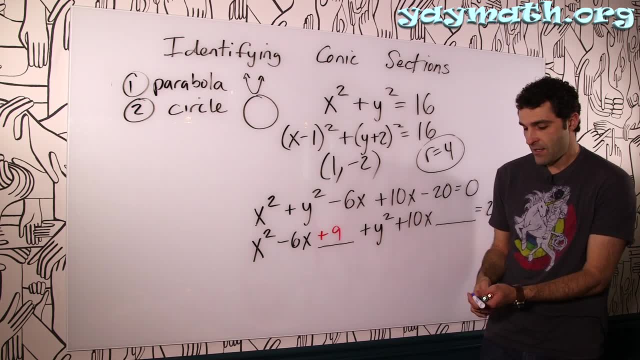 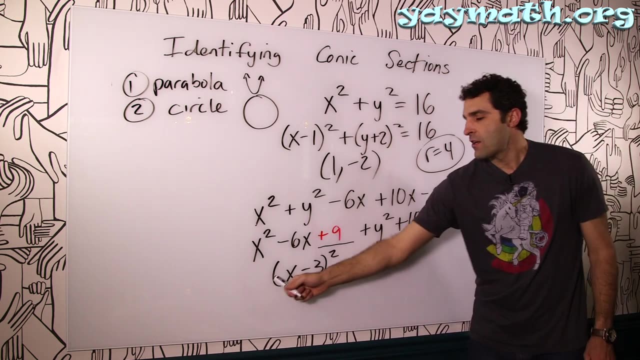 What I did before. what two numbers add to make negative six that are the same, they will be negative three and negative three. Therefore those two numbers multiply to make nine and therefore that factorization works out as follows: X minus three times itself would distribute out. 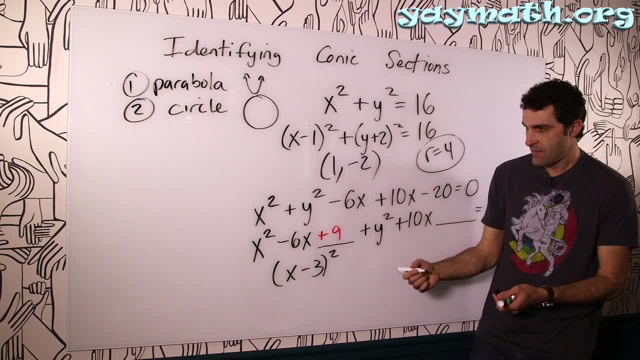 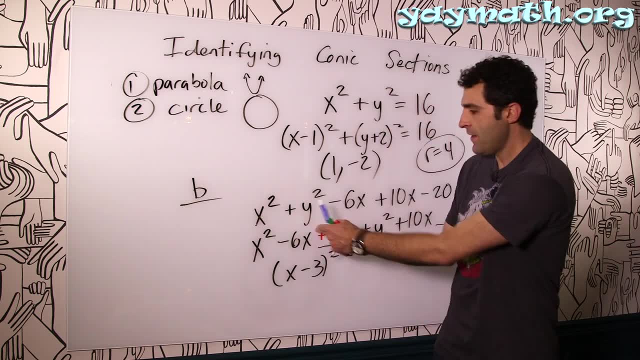 would foil out to make this. Now the process: All you do, right, All right, we're gonna do this again and again. today, You take this B value, which is B here, you half it to make negative three and you square that number. 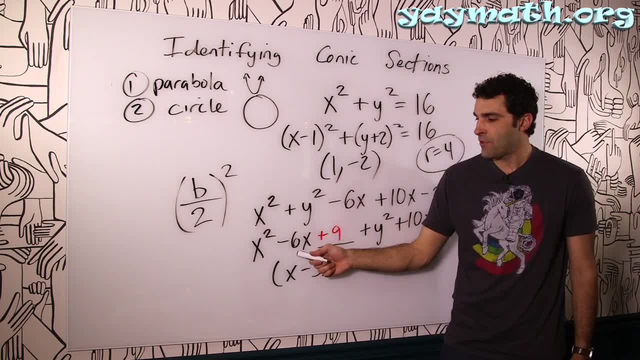 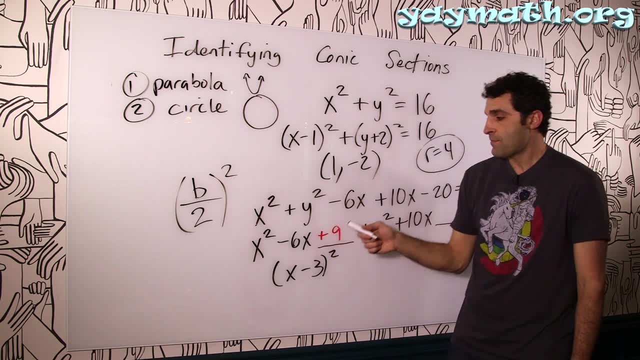 and that's your nine. okay, Again, you take whatever this value is, cut it in half. that makes negative three, and then you square it. Negative three squared is positive nine. So that's how you know what to add here. 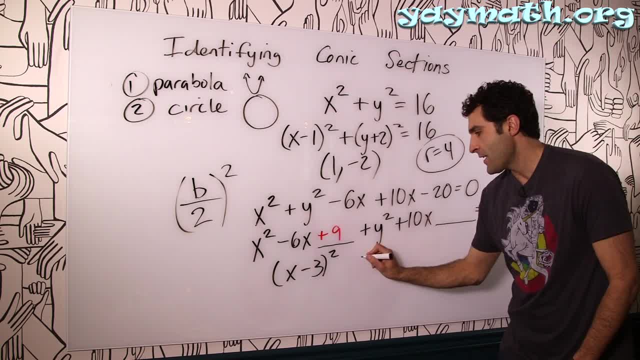 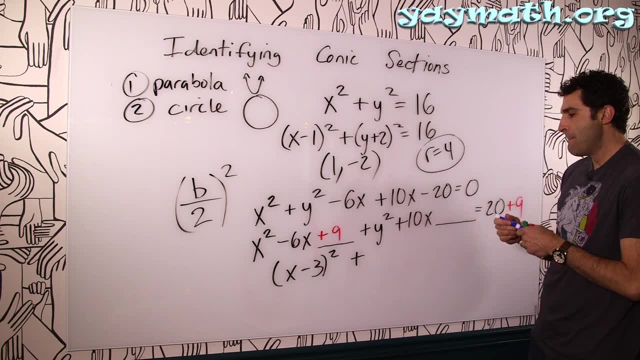 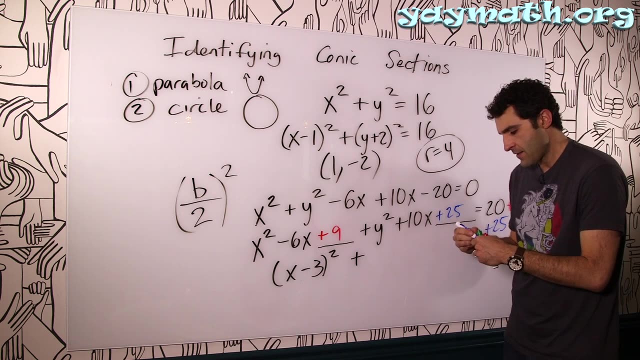 and subsequently here: Okay, let's do it again. then, now that we're in zone Half, this is five squared is 25.. Let's go: patriotic Blue plus 25,, plus 25, and we'll get X plus or, excuse me, Y plus five squared. 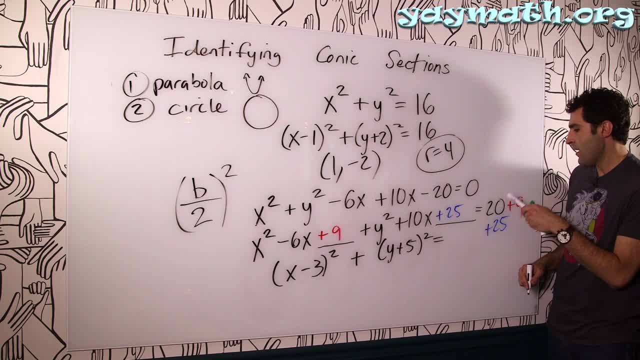 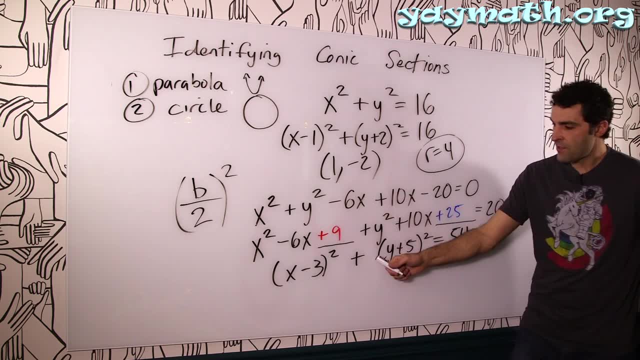 And when the dust settles, this is 25,, this is 45,, plus nine, that's 54,. all right, And so now this is a circle. We notice no coefficients. The center is at opposite three, opposite negative five. 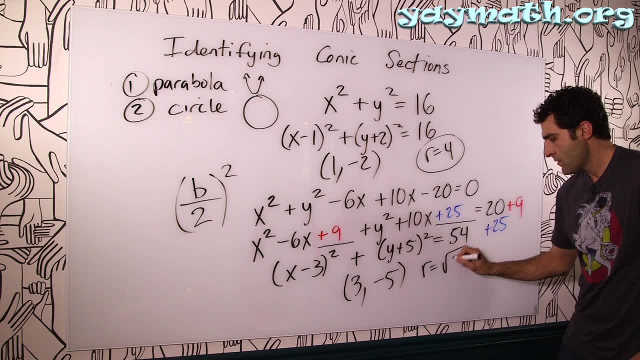 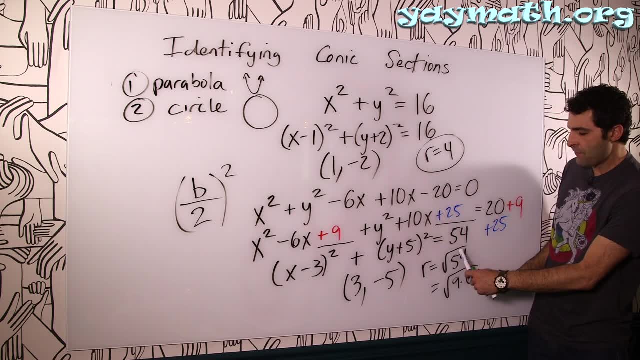 and the radius is the square root of 54,. all right, And that simplifies Nine times six is inside Nine's a perfect square hiding inside 54.. Square root of nine simplifies to the number three, root six. So there's your radius. 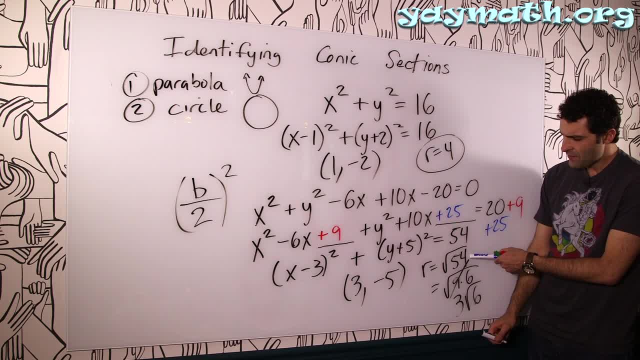 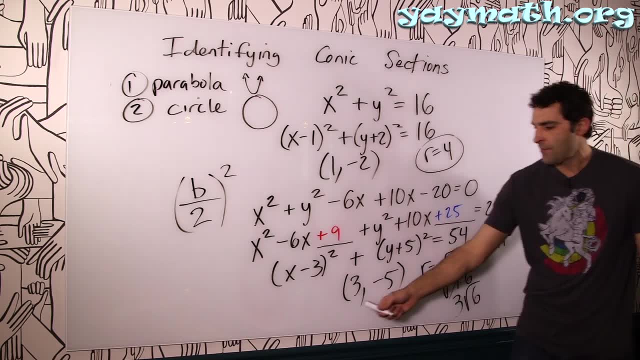 So you go up down left and right three root six, which is roughly seven point something. right, That's close to square root of 49, a little more. So roughly seven point something up down left and right from this point. all right. 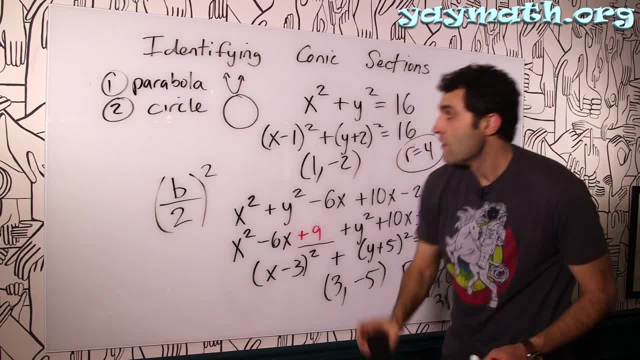 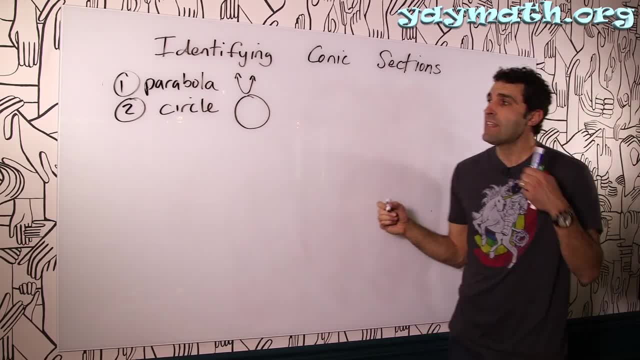 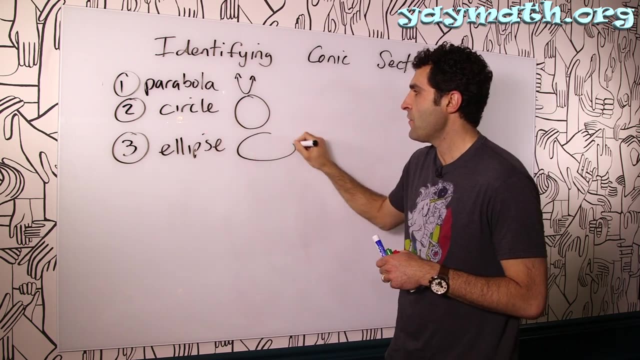 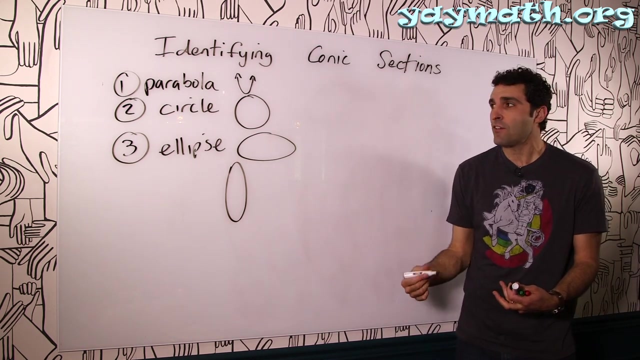 So that's the circle. Two down, two to go. Okay, next up is the ellipse. Ellipse is basically fancy for oval. all right, You could have an ellipse that looks like this or like one of these. The good news is it very much looks like a circle. 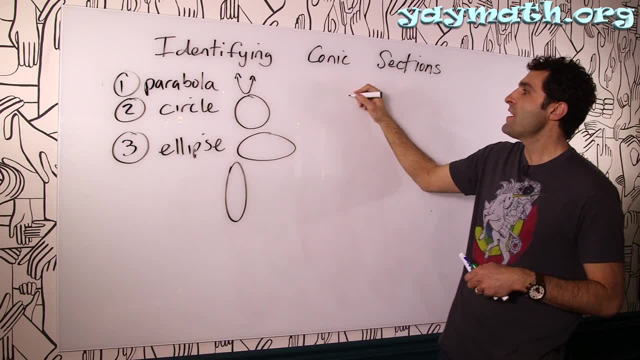 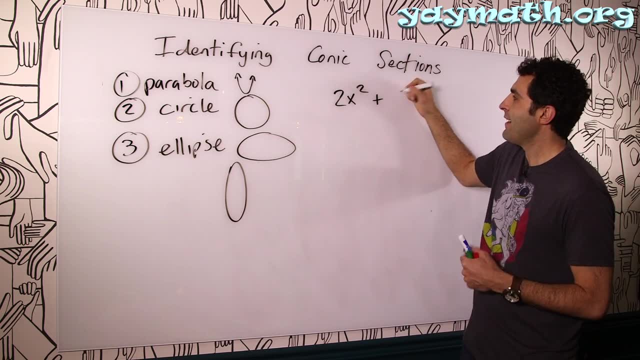 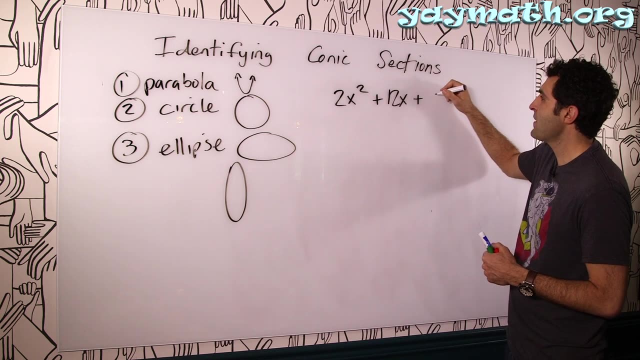 not only in shape, but also in equation, right? So you'll see the same thing going on. You'll see, let's say two x squared, let's say plus 12 x plus. see, I'm gonna mix it up today. 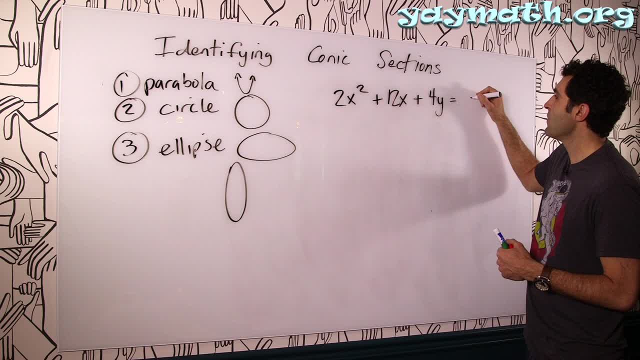 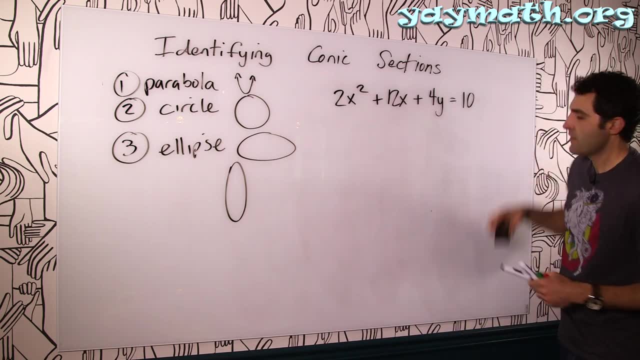 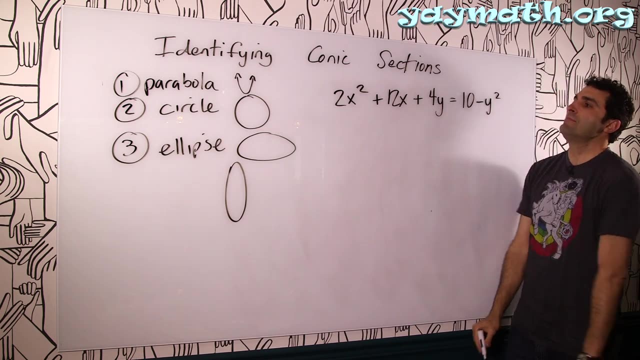 Baby, mix it: Four y equals 10 plus. how about minus y squared? This is kind of fun because you can craft it however you want. right Again, looking at this at face value: eek, right, Eek. exclamation point. 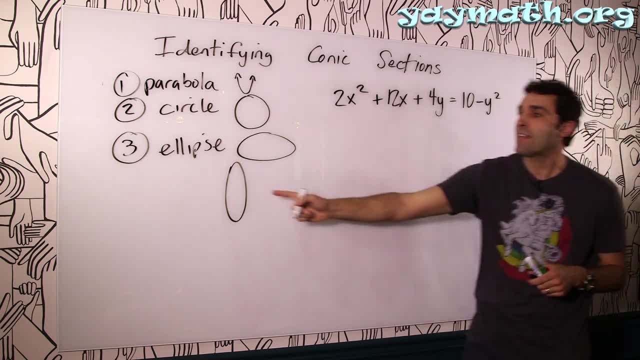 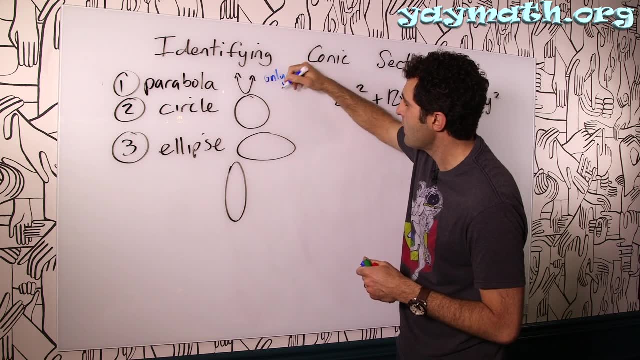 I don't know what this is. I don't know how to identify, until you recognize that, the ellipse. why don't we make a few notes here? Few notes, Only one variable squared. That's good. Here you have both. 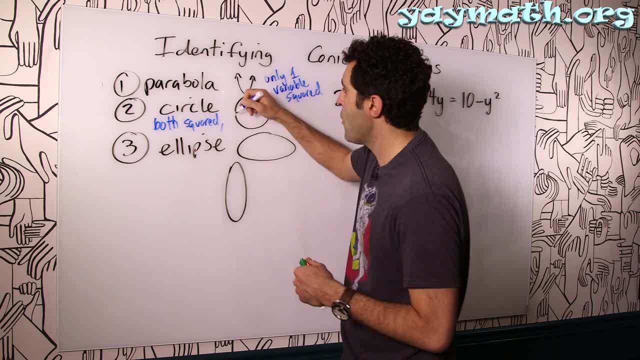 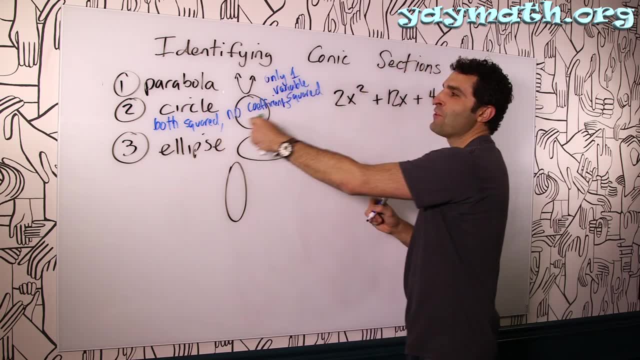 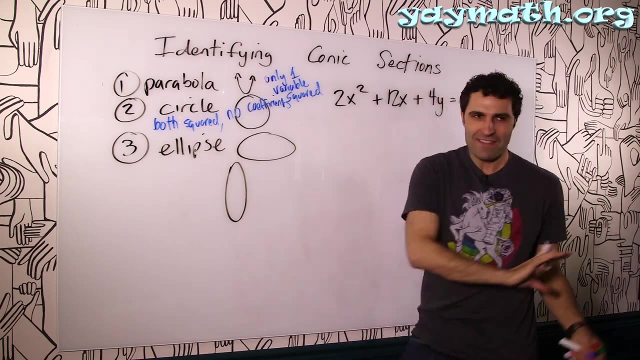 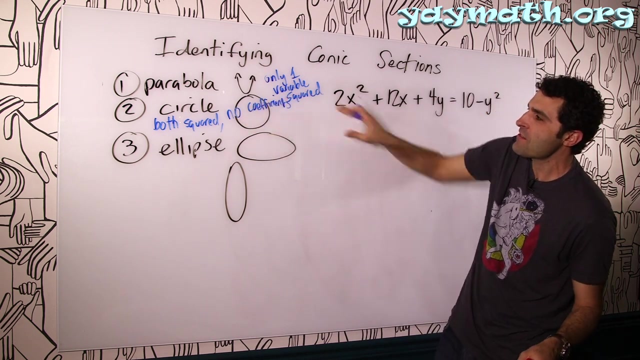 squared. No co- efficience. Looks like the Universal logo: Hollywood California Instead of Universal. it's like no coefficients And that's like the scary music from the movie, Like an alien movie in black and white- No coefficients. 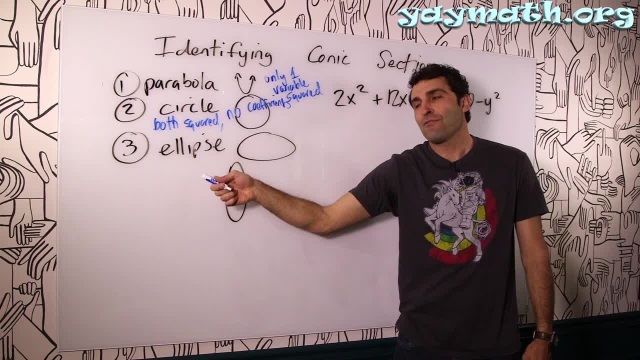 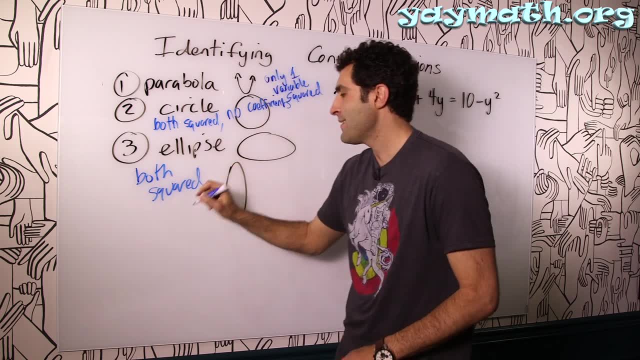 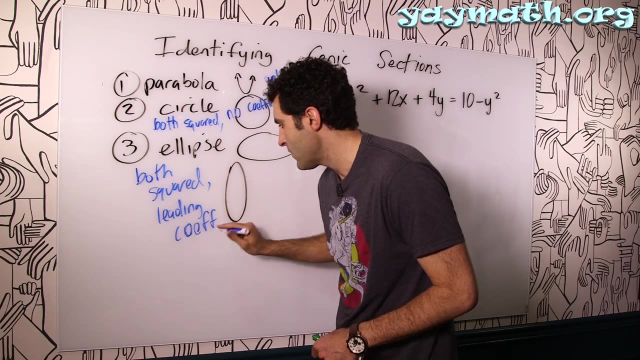 Which isn't scary at all. actually It's very inviting. But the ellipse does have coefficients, So again, it's both squared, Both squared And leading coefficients. Look, don't let the vocab mess with you. This is a leading coefficient, that's all. 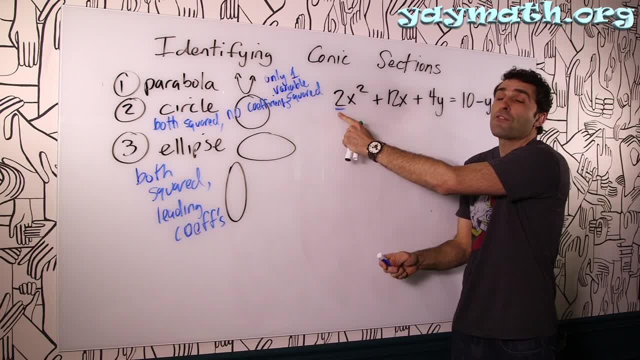 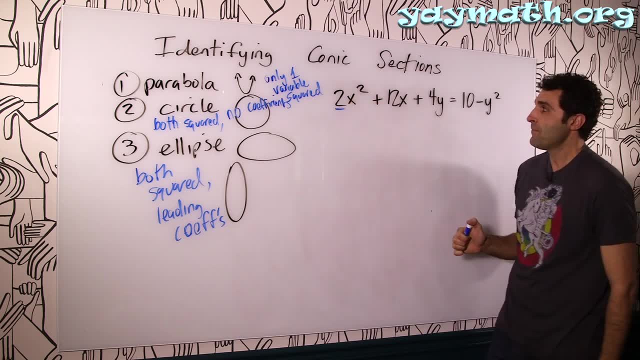 It's the number in front of the squared value. That's other than one. All right. So it's a leading coefficient. that's not one That the circle did not have. This does have it, Okay. And then we have like, oh well. 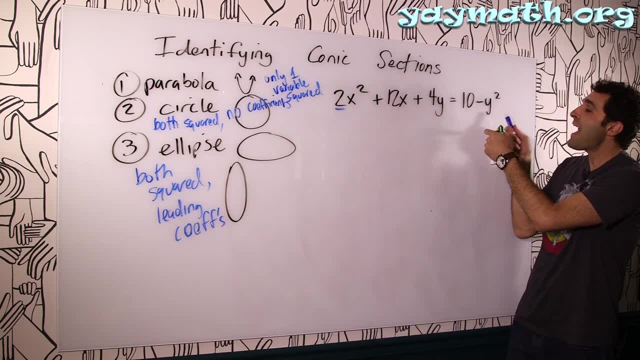 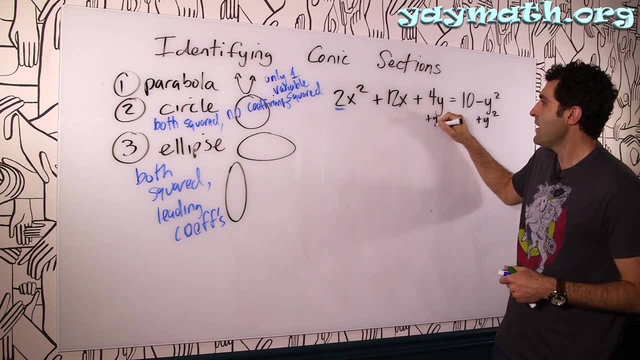 how do we prove that both variables are squared? Oh, here we go. If we add y squared to both sides, then that proves it. If we go plus y squared, plus y squared over here, then we prove that we have our x squared plus y squared. 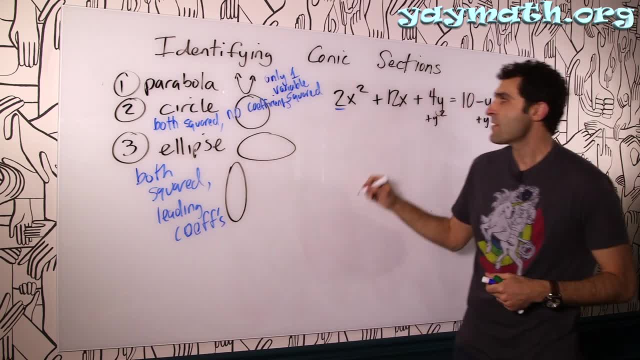 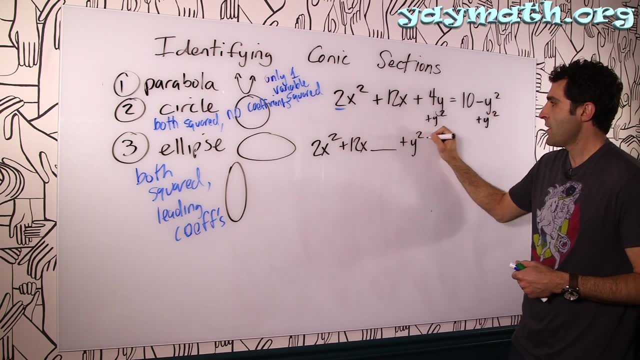 on one side of the equals. So this is indeed proving to be an ellipse. Let's go ahead and group Two x squared plus 12 x. Leave a space. Plus y. squared plus four y. That's fine, Leave a space equals the number 10.. 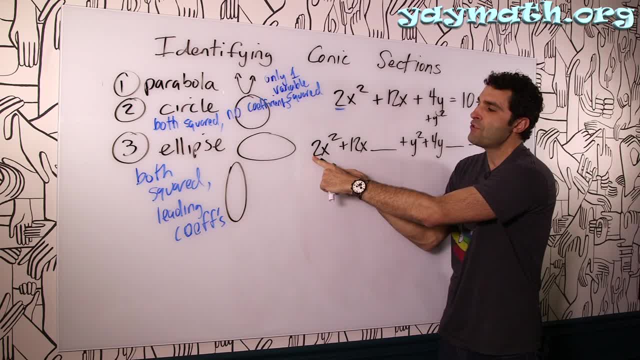 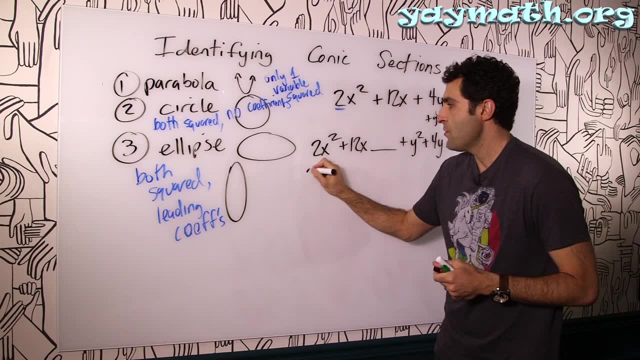 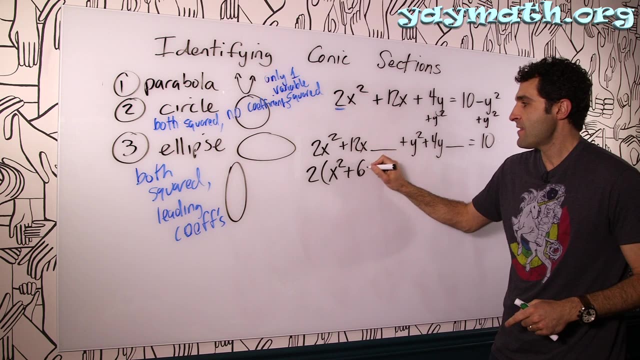 All right, To complete the square here, we first must factor two out so that we have a isolated x squared term. Here's what I mean: Two comes out X squared plus two times, what would result in 12 x, That's six x. 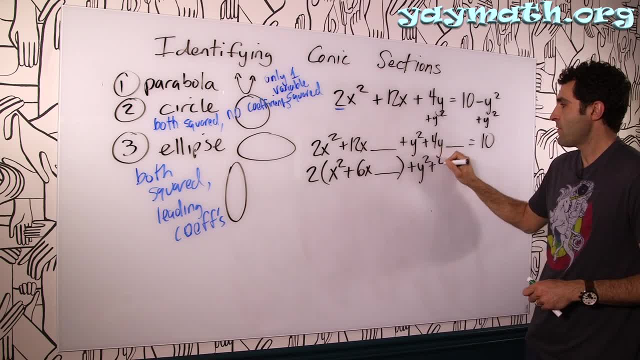 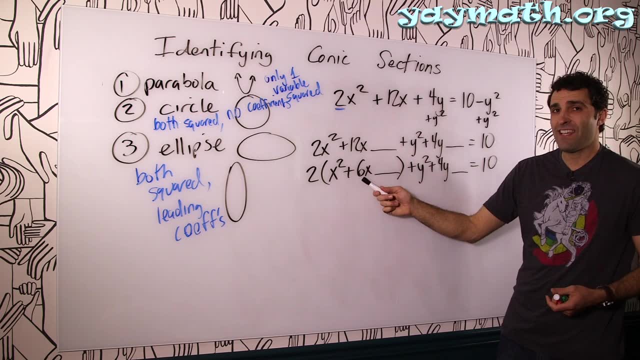 Still leave a space Close Plus y. squared plus four y Leave a space equals 10.. Now we can complete the square. All right, Half of b, half of six is three, Squared is nine. So add nine over here. 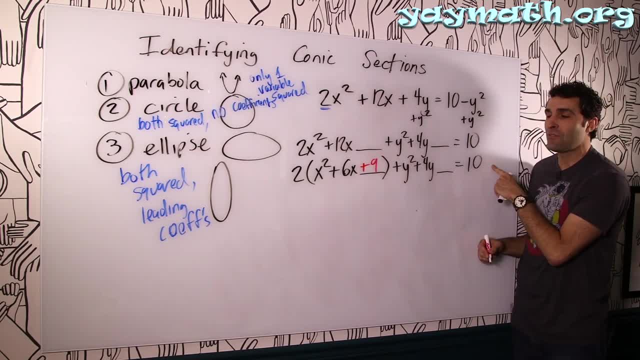 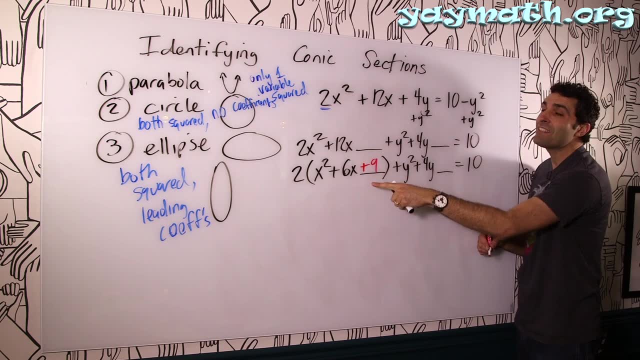 And now the temptation that a lot of students have is to add nine over here too. They're correct in spirit. In theory they're adding nine, meaning they added nine here, But the issue is we really didn't add nine to this side of the equation. 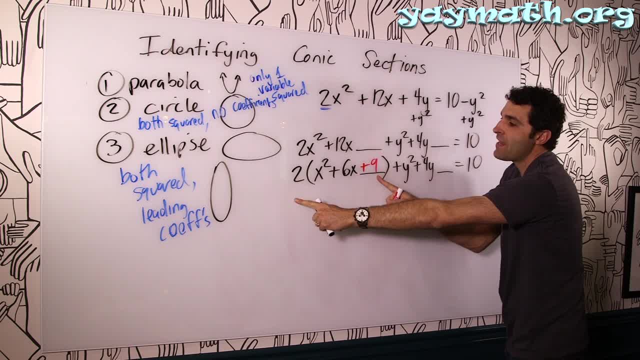 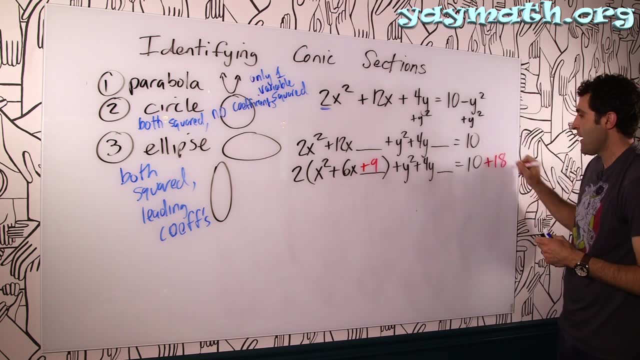 We added 18 to this side. We added 18 to this side. We added 18 to this side of the equation because the nine is affected by the two's distribution. So this would have to be plus 18 over here, All right. 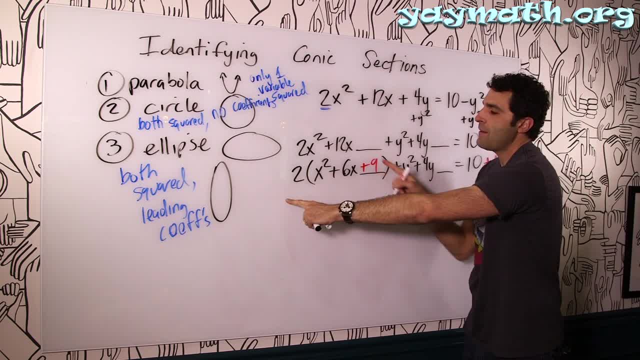 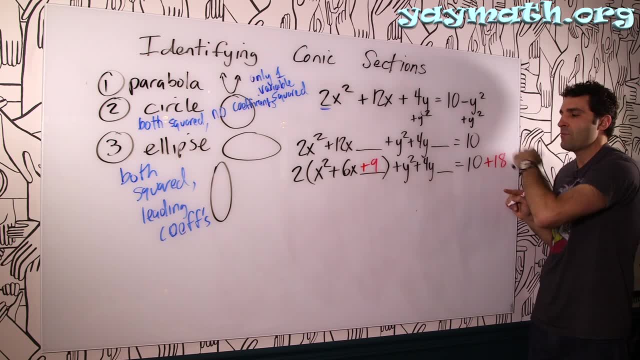 I trust that you can remember that. okay, Just look at it here. Two times nine is really 18.. So it's a really a net change of 18 to the left side. Thus, to counterbalance, we add 18 to the right side. 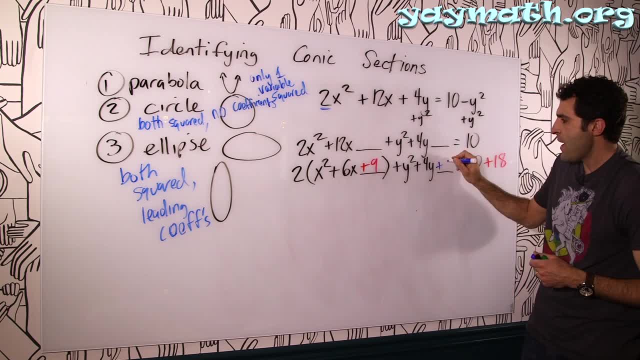 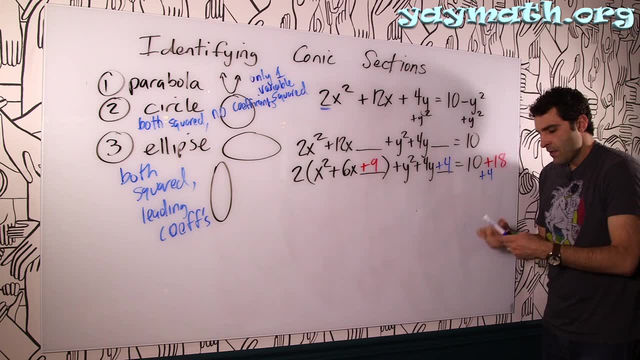 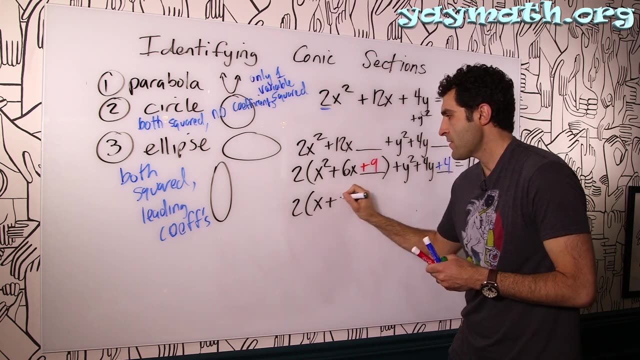 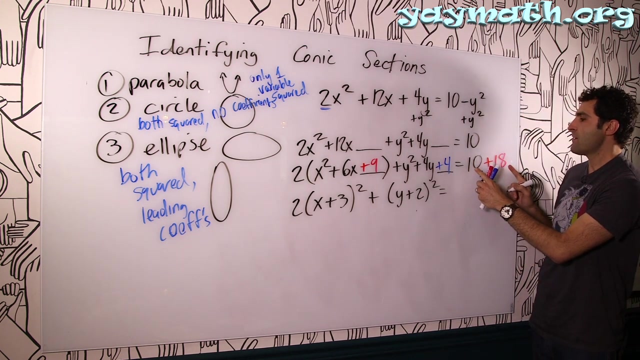 All right, Continuing, our America colors America Plus four. half of this squared is four Plus four. Good, Now we're going to factor. So this is two X plus three squared plus y plus two squared, equals: this is 28 plus four is 32.. 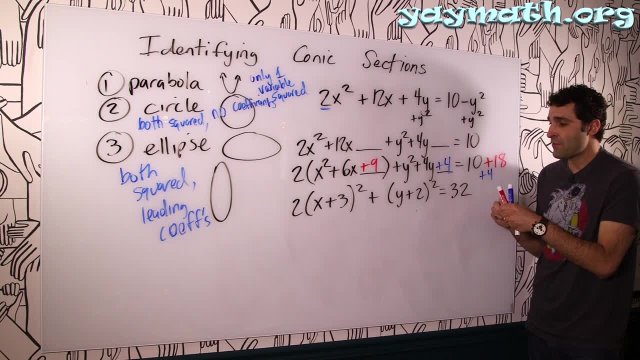 All right, And then we have our ellipse. Technically, the form for ellipse, the standard form, now that we recognize coefficients out here, is to set this value to one. You'll see that in the books. Once it's no longer a circle, once it's like loses, 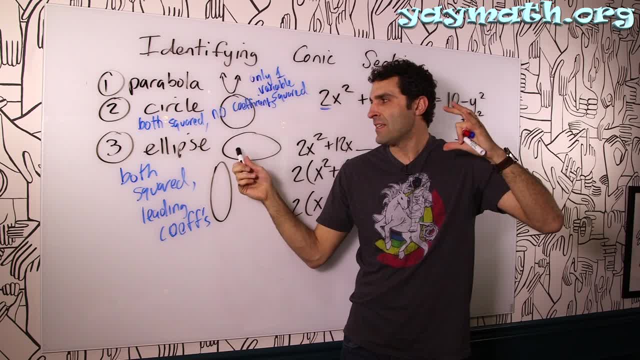 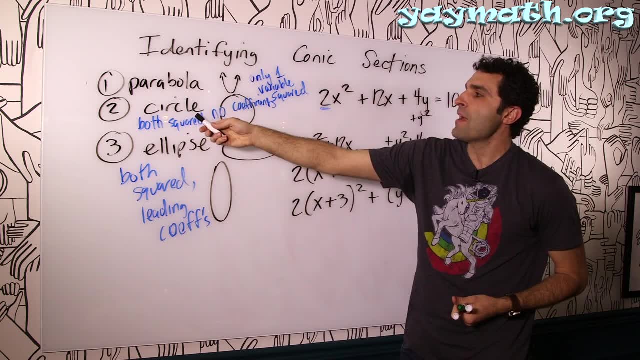 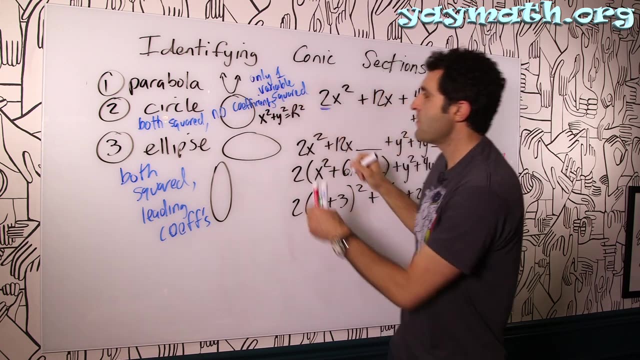 it's like a symmetry. Well again, ellipse is symmetric, but not completely, Once it loses that perfect round shape and becomes wide, like this. you step away from the x squared plus y squared equals r squared thing. Right. You step away from the thing we did on the last problem. 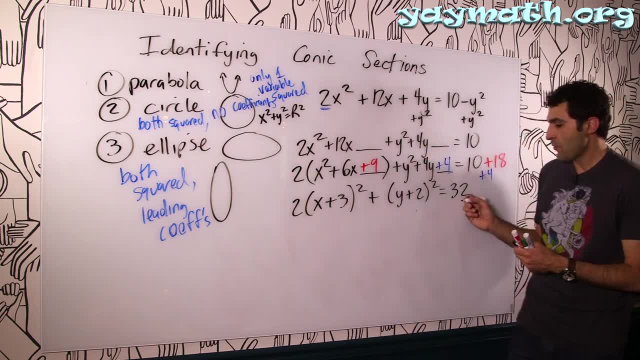 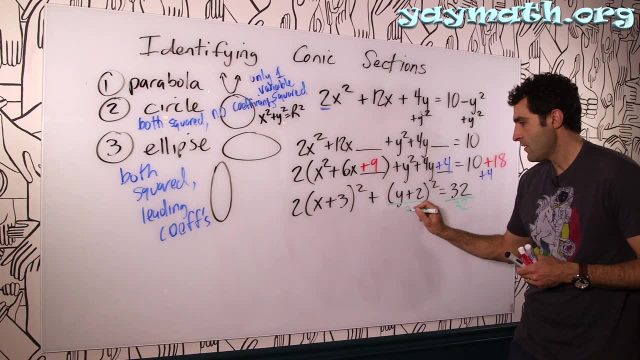 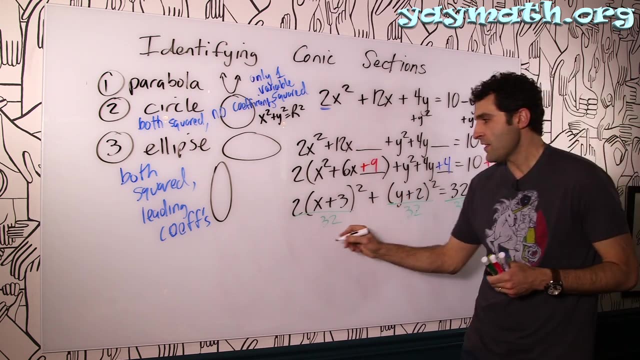 And you set this to one To help you graph. In order to do that, all right, let's go green And divide by 32, here, here and here. So now we'll get the ultimate equation, the standard equation of ellipse. 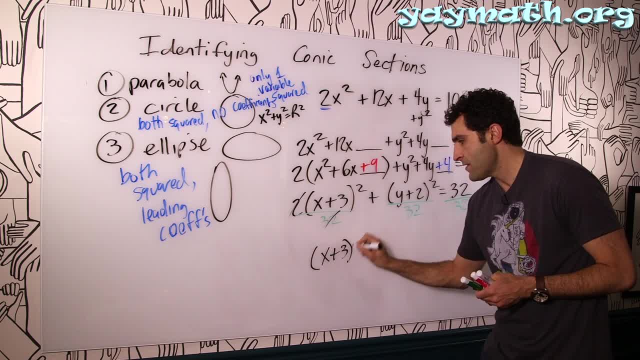 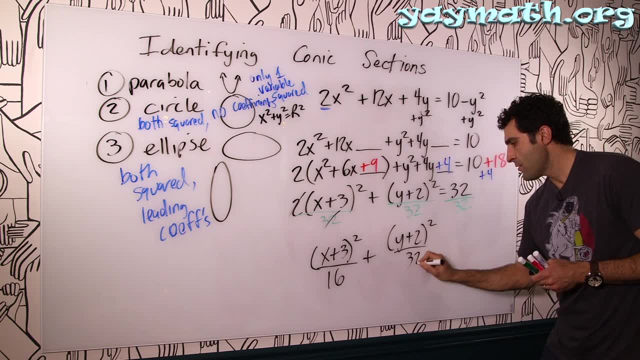 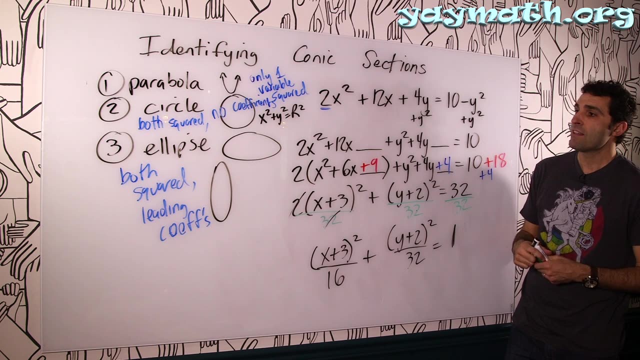 Two and 32 go away, leaving 16 x plus three squared over 16 plus y plus two squared over 32 equals one. So there's your standard equation of the ellipse. You'll notice the giveaways are: both are squared, There's a plus right. 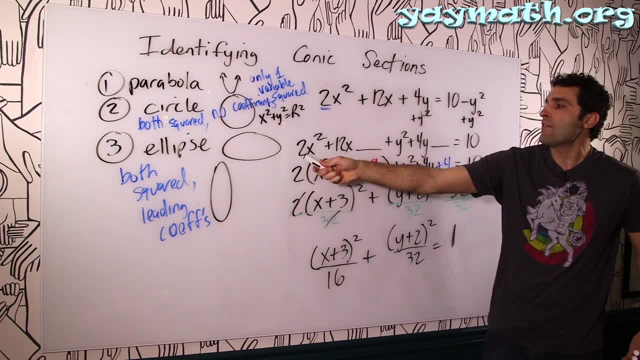 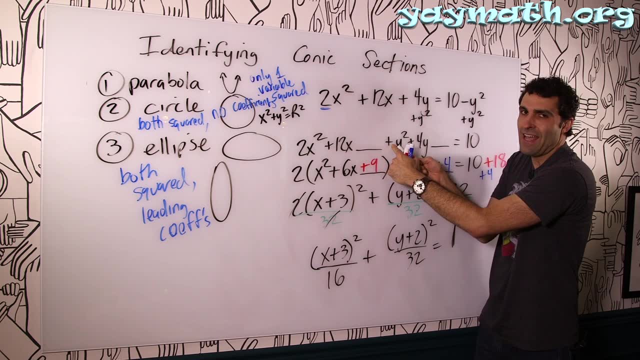 X and y are squared. There's a plus between them. You have leading coefficients in front of x and not in front of y, right, If it was a two here as well? that's sort of a sly little trick. If both were two, you would divide them both. 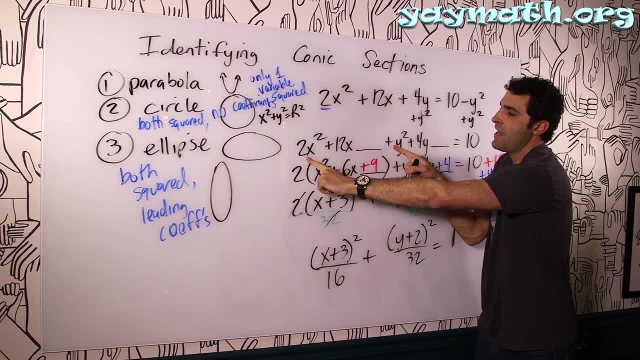 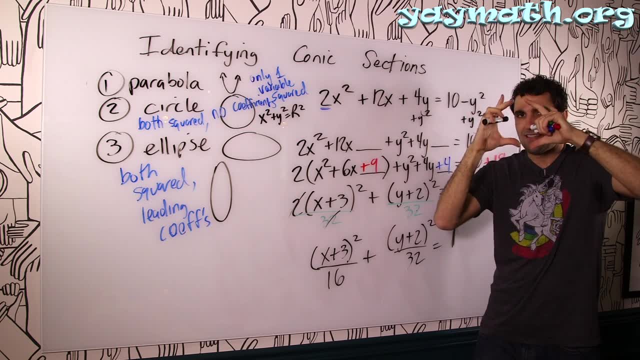 and then they'd both be going away. But if you see that they're not the same, then that's the giveaway: That what started as your circle is now weighted- Weighted in terms of x, right, So you get this like little ripple effect on the circle. 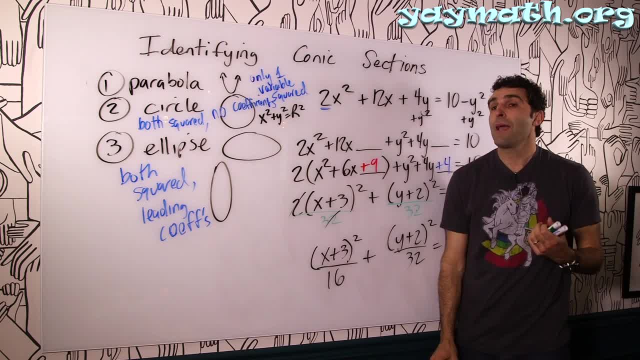 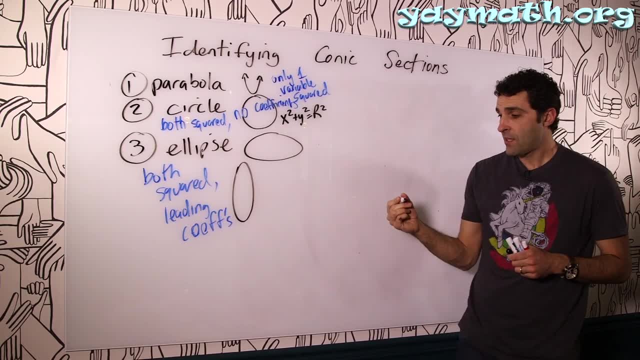 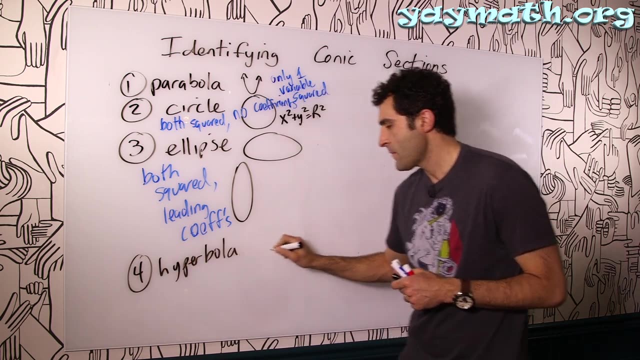 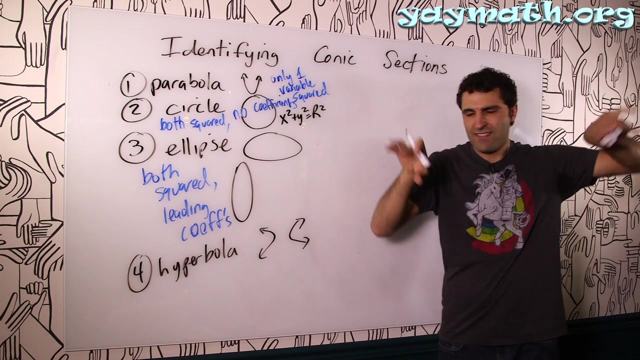 making it an ellipse, Let's do the hyperbola next. So with the hyperbola you have hyperbola. That's one of these Somewhat parabolic shapes Just facing outward from each other. You do have upy downy as well. 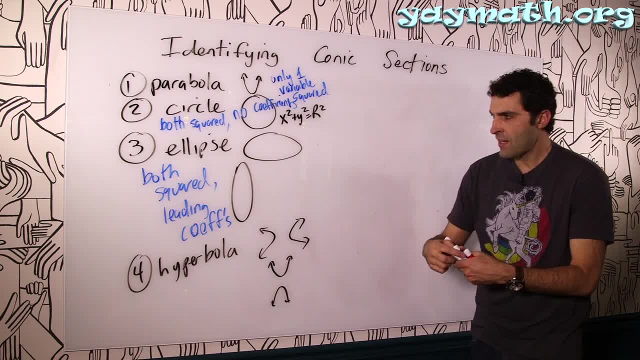 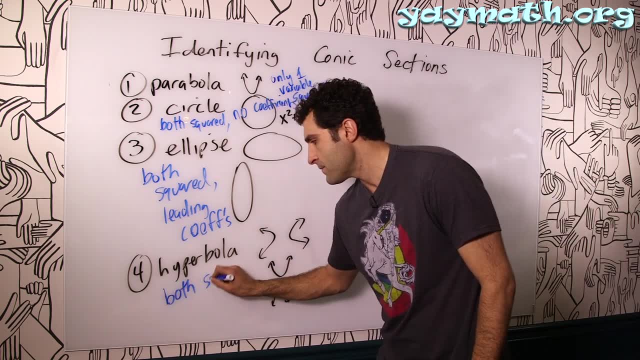 Here you go, you have those, Okay, And so there's a sort of a neat trick that I- at least it worked for me, it occurred to me- You still have both squared X and y squared Right, To confirm the only one in which one was squared. 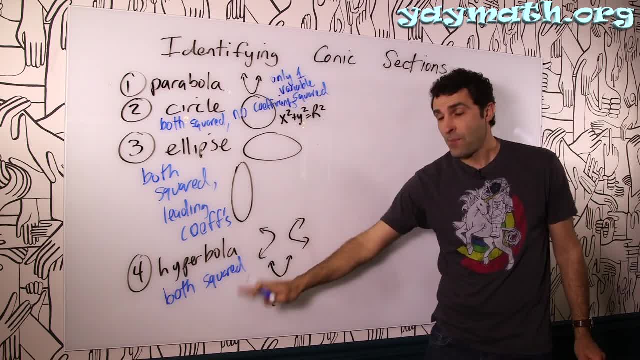 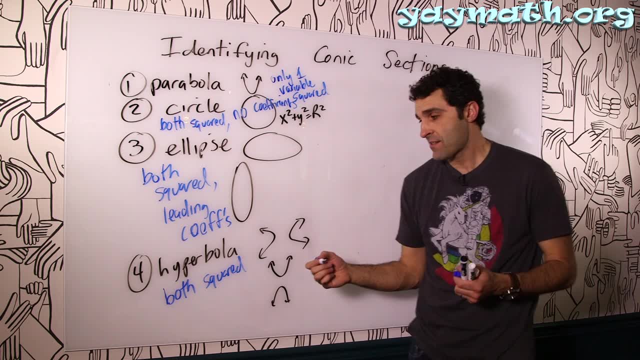 was the parabola. The rest of the three- x and y- were both squared, But now you don't have a plus between them. Between the two you have a minus. Right, It's x squared minus y squared. 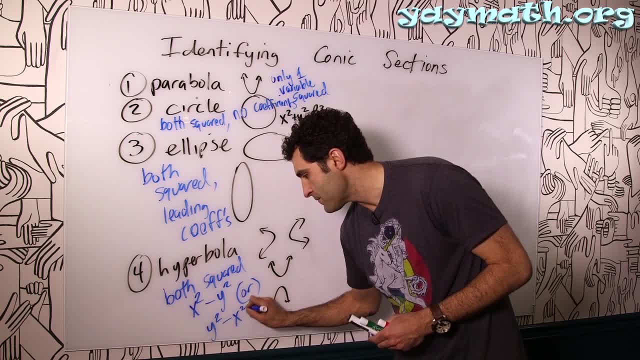 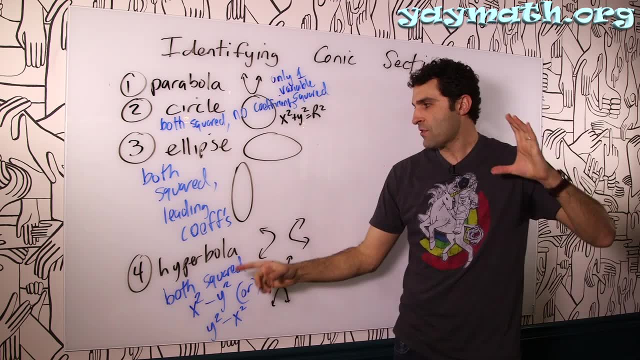 Or y squared minus x squared, And what that makes me think of was, like what started with x squared plus y squared, what started as plus between them was this harmonious shape where it's like plus, You're adding the two pieces together. 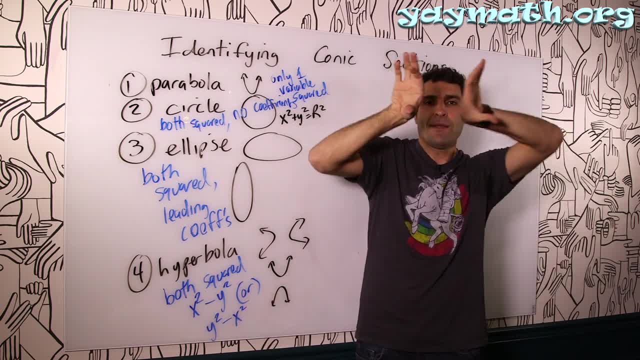 Whereas if you have minus between them, it sort of ripped it apart and made it go like that. Even the ellipse had a plus between them. They were still. they were working it out. They were like: okay, I'll meet you in the middle. 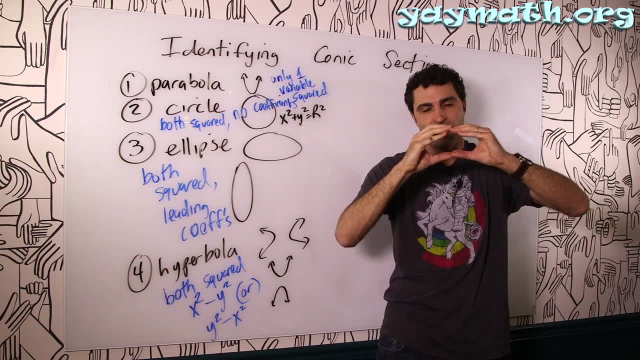 I'll like: we're a little weird. we're a little weird, but we've still got harmony. We're still an oval, a circle. We can go around and around and around. But the second you put a minus, a little negativity here. 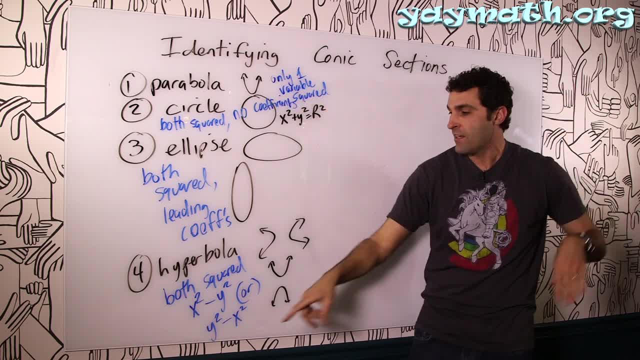 rip apart. I'm not even gonna look at you anymore. We're not looking, we're not looking. Okay, So the second. you see a minus between the two squared immediately hyperbola. that's the giveaway. That's all it is. 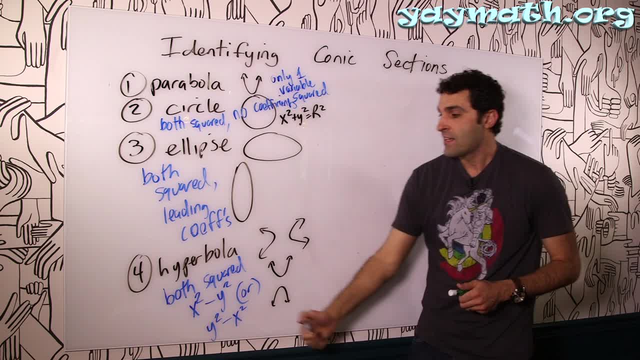 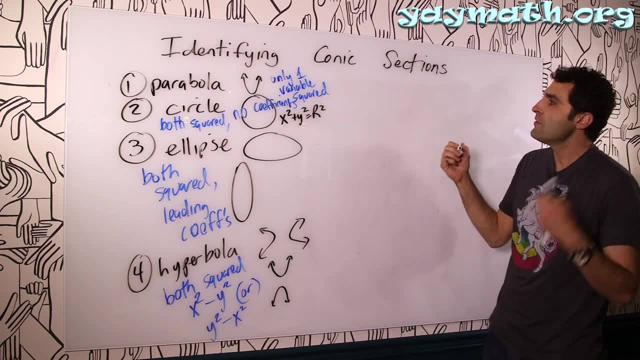 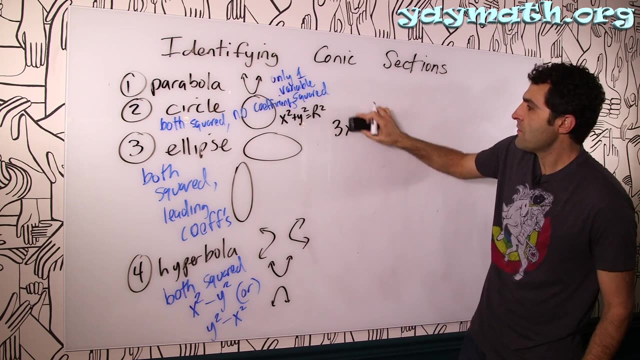 Regardless of coefficients. Regardless of coefficients, right? So even if there's coefficients, but still minus 100% hyperbola. Let's give a brief example with coefficients. Let's go with three x. we can even start with y squared now. 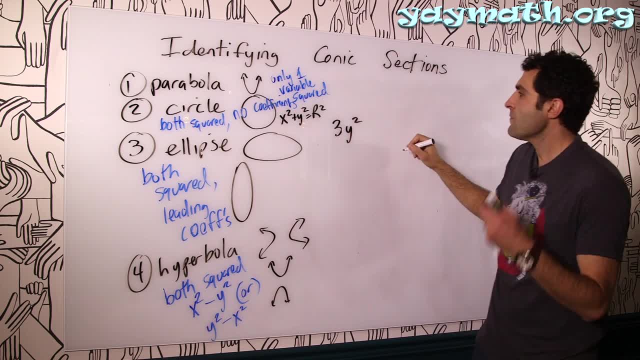 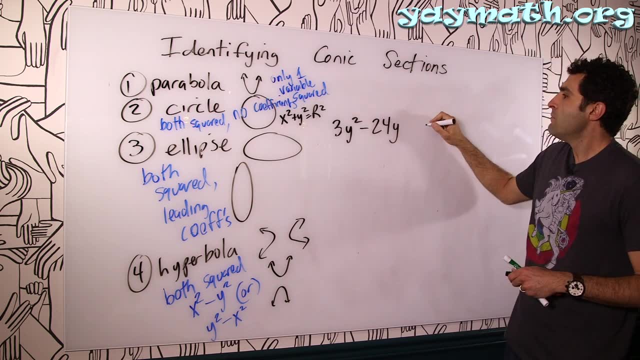 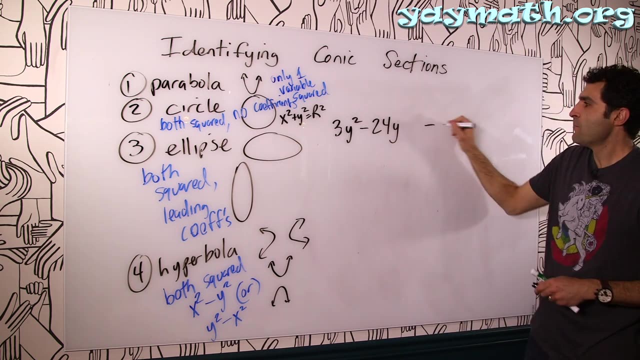 You know, mix it up a bit. Three y squared plus say minus 24 y Plus whoa, minus Minus, right? I'm much more of a believer in harmony, So that's why I did the plus. 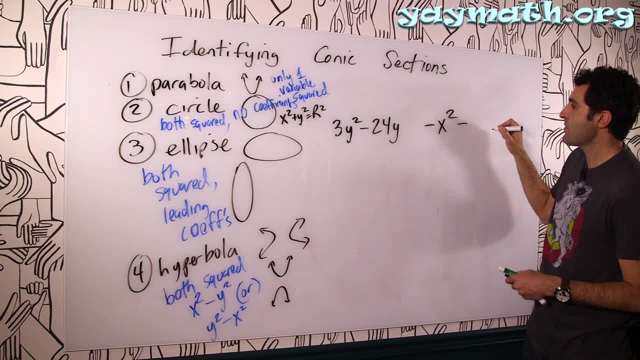 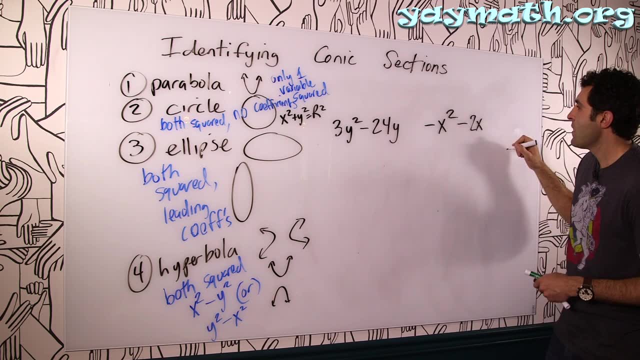 X squared. let's go with ooh minus. This'll be fun. Let's go with two x And then we have equals. pick a number at random. Let's go five, won't matter, right? Whatever, the problem is. 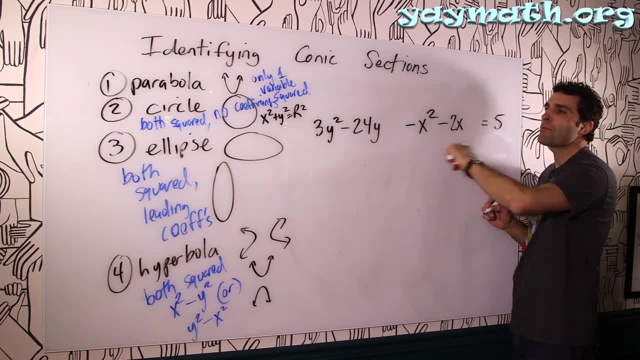 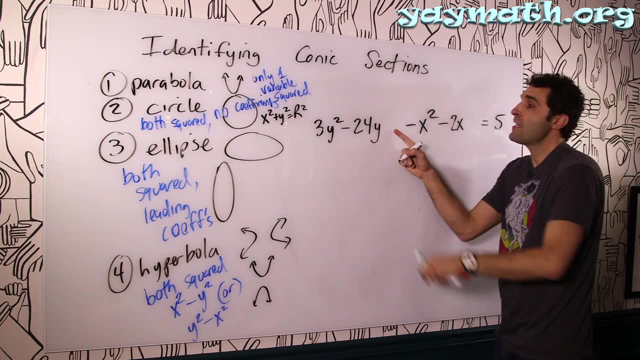 So you'll notice, I've already gotten to the habit of arranging right, So the problems will be presented in different ways. But now, since it's our fourth conic, that's where we got together. You can see, I'm already arranging. 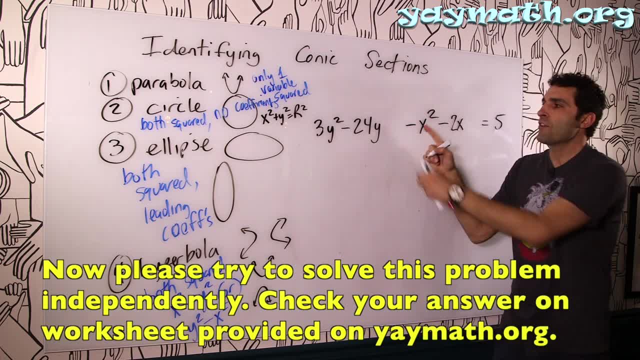 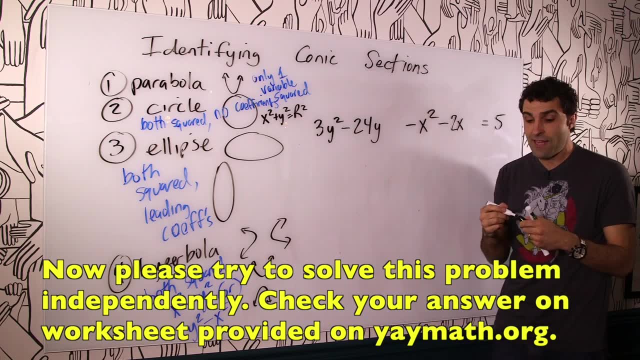 you can see I'm already leaving a space here, So you're invited to do the same thing. You're gonna group your y's. you're gonna group your x's. put the number on the other side, complete the square and then you'll be set to go.